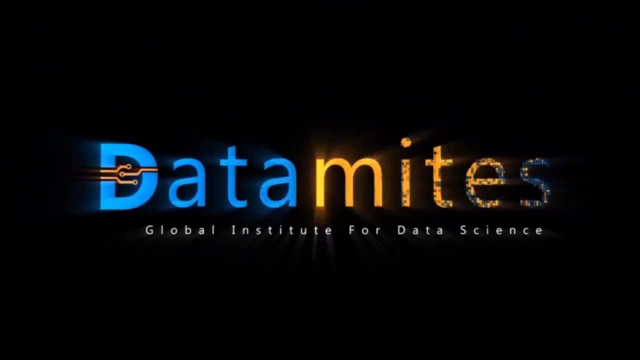 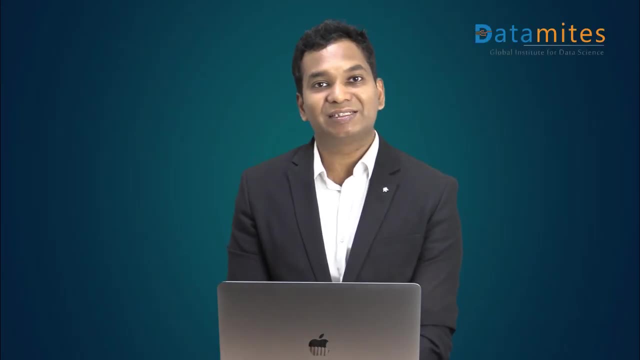 Hello everyone, I am Ashok. Today's topic is ROC and AUC score. ROC stands for Receiver Operating Characteristic and AUC area under the cup, And these are very important metrics for binary classification. To understand the purpose of this, let's first take an example. 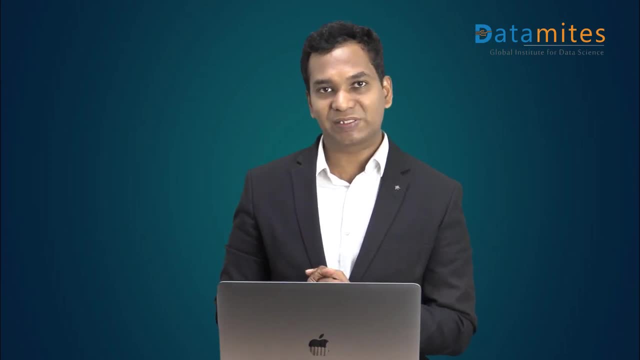 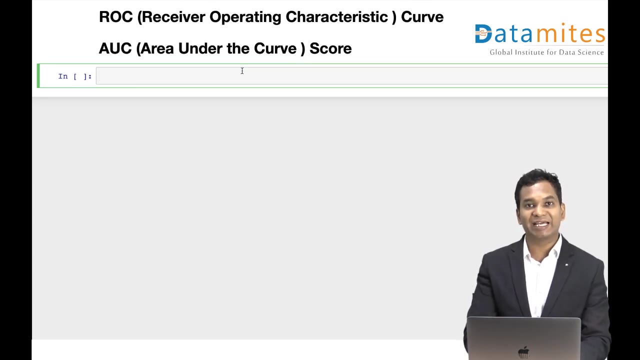 understand the binary classification itself, and then we will go into ROC and AUC. So I'm going to use one of the standard data sets: breast cancer data sets from UCI repository. Importing pandas Data is equal to BCSD- Breast cancer data set. Let me print the: 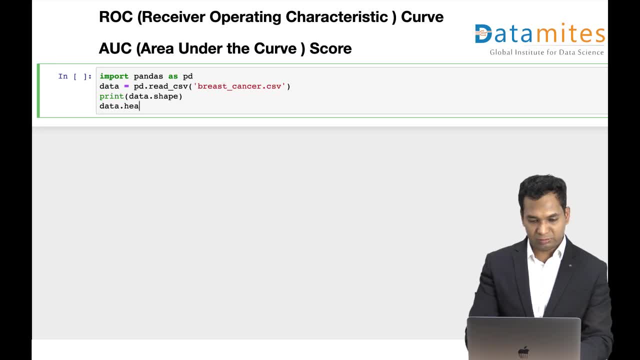 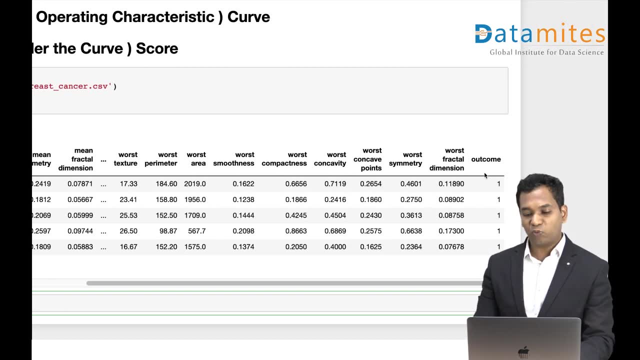 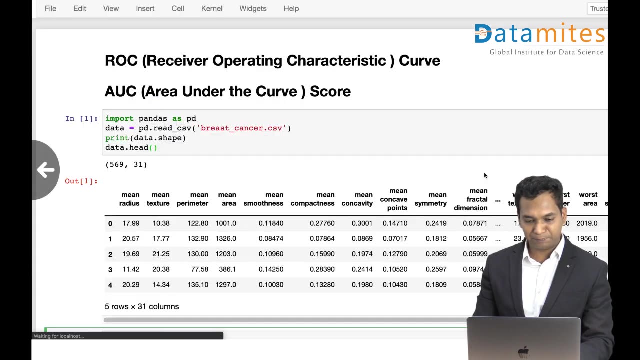 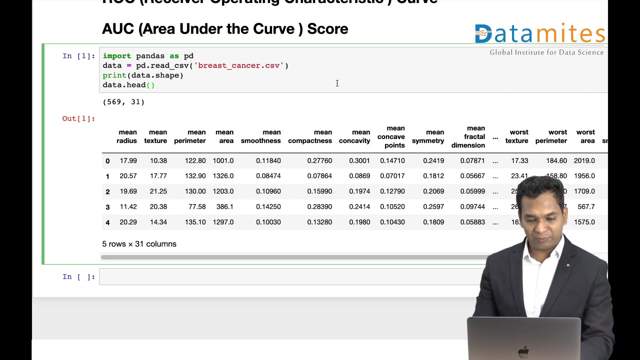 shape of it. So this has 30 columns as a predictors and the last one is outcome Outcome. one means diagnosed with cancer, malign, and zero is no cancer, which is benign case. Okay, So for this example, I'm not. I'm not going to use all the 30 columns as my predictors. 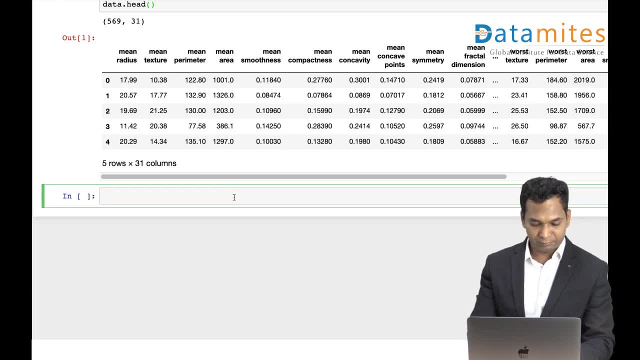 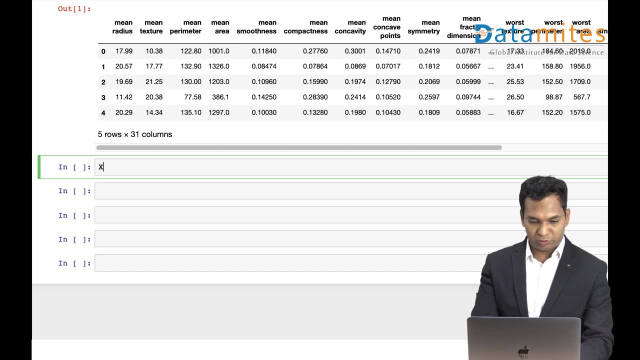 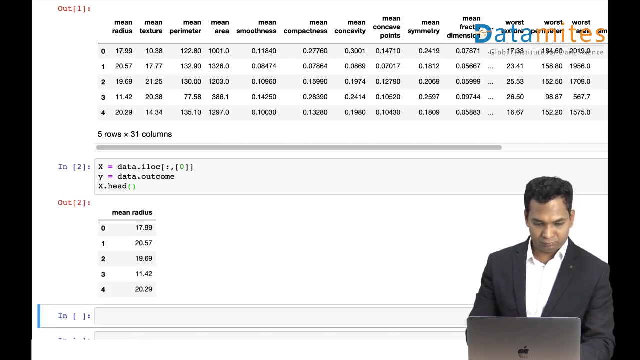 I'll be using only one column for simplicity sake. So I'm going to say X is equal to data ILOC- All the records, only the first column, Y, is equal to data outcome. Okay, So that's my X, and Y is equal to data outcome. So that's my X, and Y is equal to data outcome. So that's. 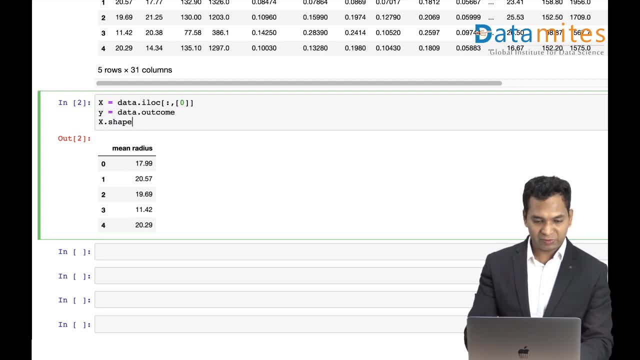 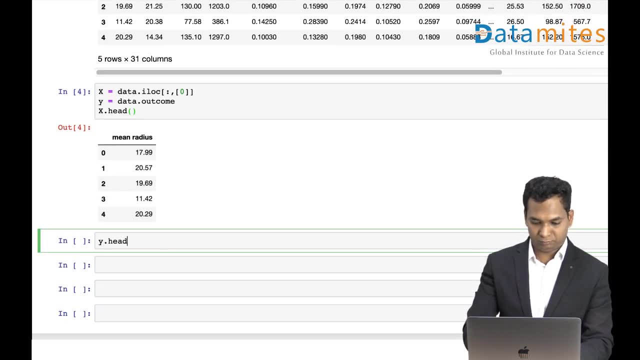 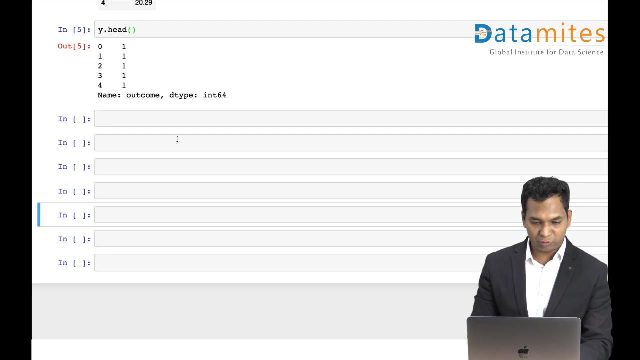 my X and Y would be. let me also look at the shape of the X. Yes, Pretty good. Y is your outcome, All right, great. So, um, let me quickly spam me a minute. I'm going to quickly build. 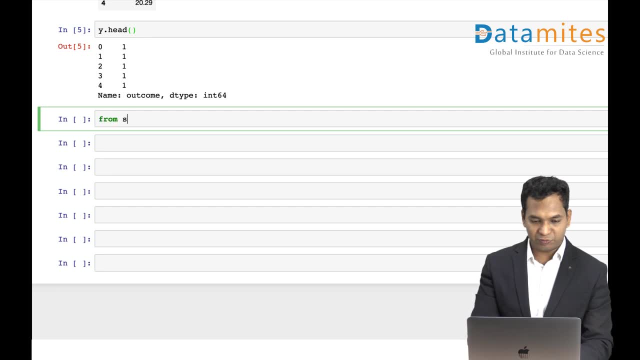 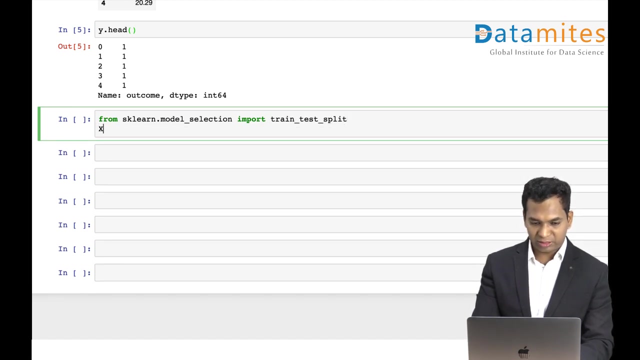 a logistic regression model. So for that I need to first of all, let me first split the data set. uh model selection, import train test bit and I'm going to say X, train, X test, Y, train test equal to train test bit, X, comma Y. 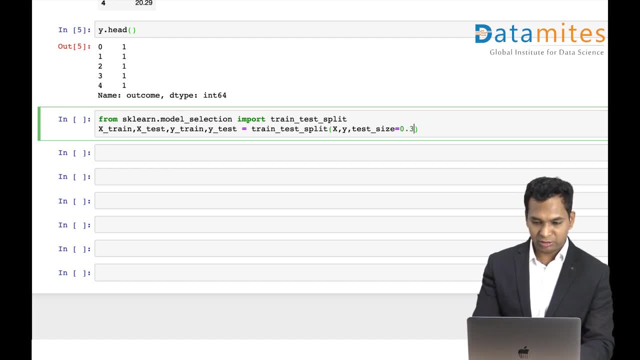 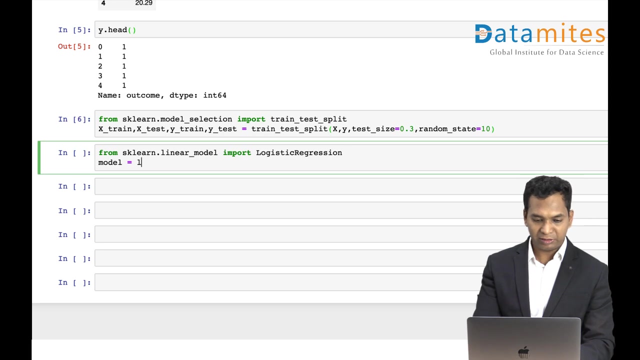 I'm gonna put a test size as 0.3 and random state, as I always put some time great. and then I'm going to import logistic regression model. it's in your linear model package. import logistic regression and say: model is equal to logistic. I'm not gonna do any fine-tuning here. the purpose is not. 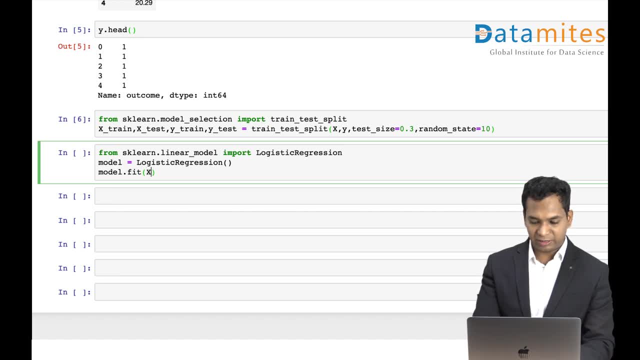 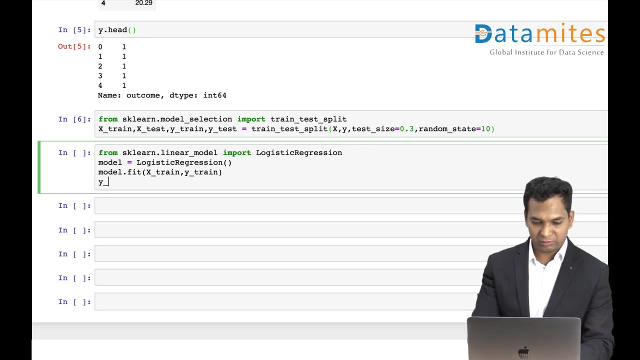 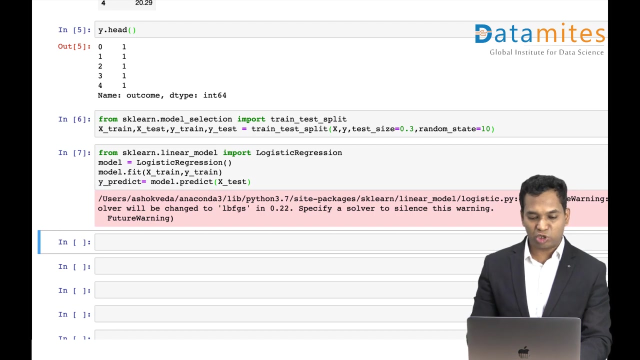 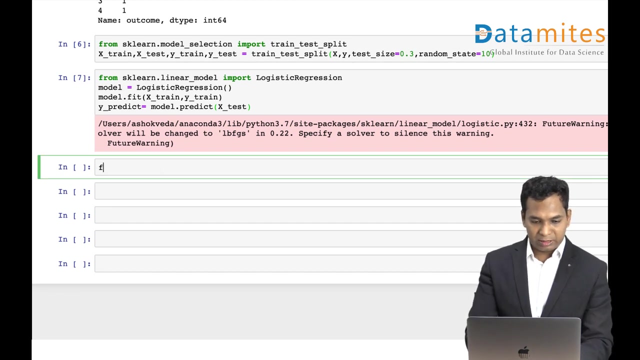 modeling. say fit fitting X train, Y train, and I'm going to predict, is equal to model dot predict X test. so training and prediction is done. ignore that warning. it's a future warning that a default solver is being replaced with LBF DS next version. so evaluation from matrix: import- I'm going to import. 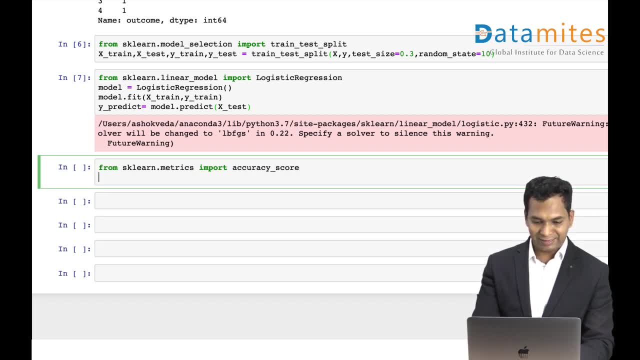 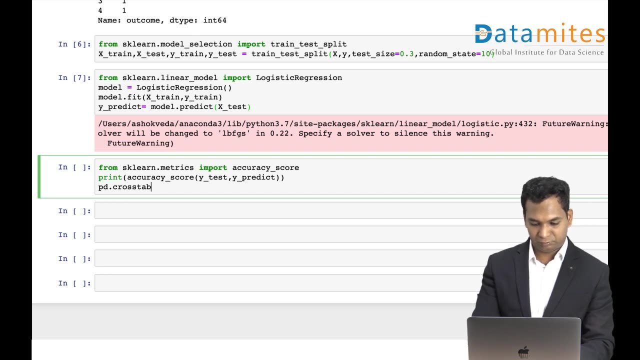 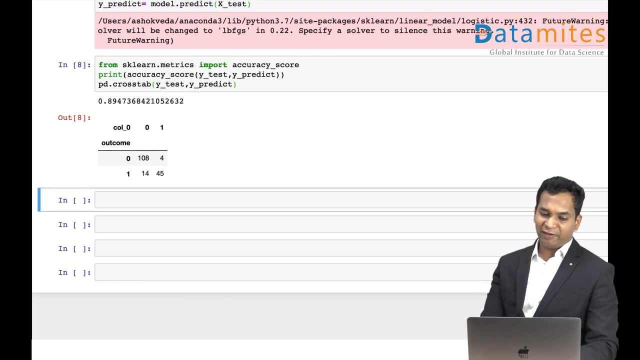 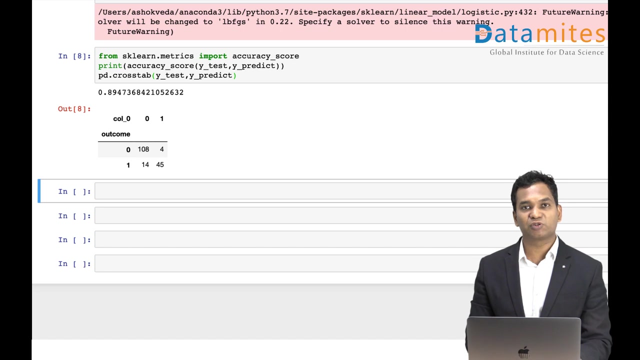 accuracy score. I said accuracy score and print that accuracy score: y test y- okay, and PD cross tab: y test y- great. so we have about 90% accuracy with just single variable. if you actually take all the variables you, you will reach close to 100%. 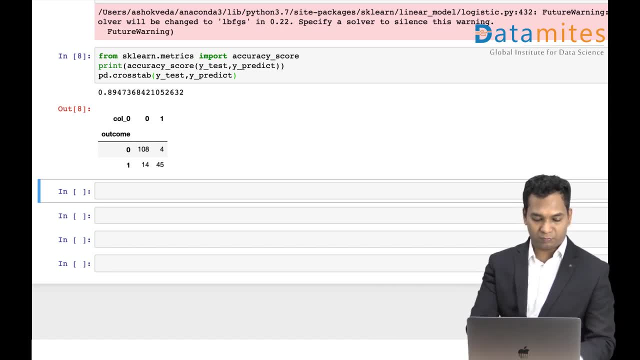 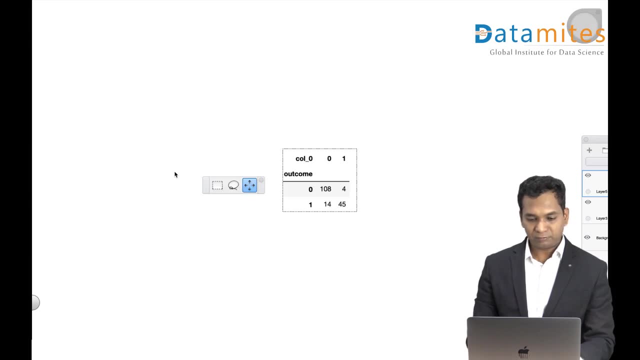 accuracy. but this is, if you really look at this. this is confusion matrix. I'm going to explain it on a very high level. I have a complete video on confusion matrix- we can search in the same channel- and patient matrix, and that explains configuration matrix in much more detail. so for now I'm going to take a quick. 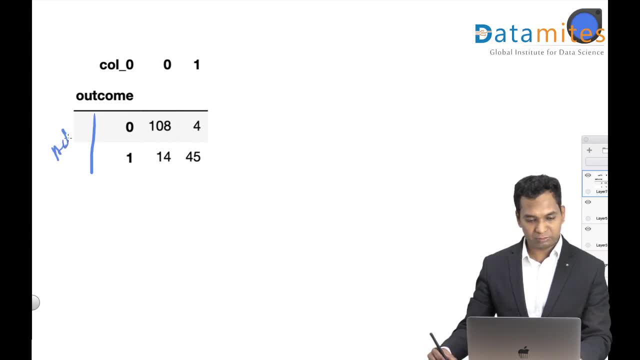 explanation- this is actual and this is what we're going to do- is we can query the configuration matrix. we're going to look at the configuration matrix now. we can look at the configuration of the matrix by using this normal set of everyday variables. now, here's what we've come across. this may be the case that we 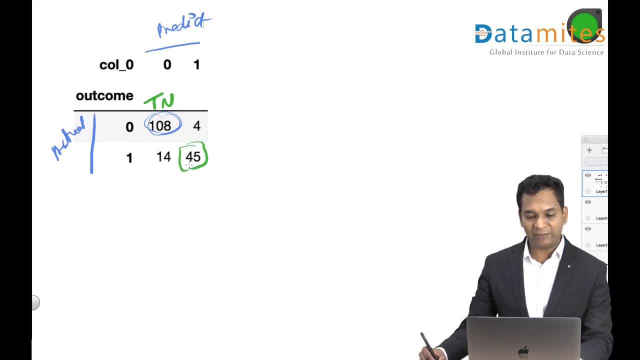 slightly skip this, but I think it makes a significant difference because when we look at this configuration matrix, you really see that it's fairly straightforward. every single variable is here, if you look at it, from the signal model and from the, and this four are non-cancer being predicted as cancer. this called as false positive. these guys. 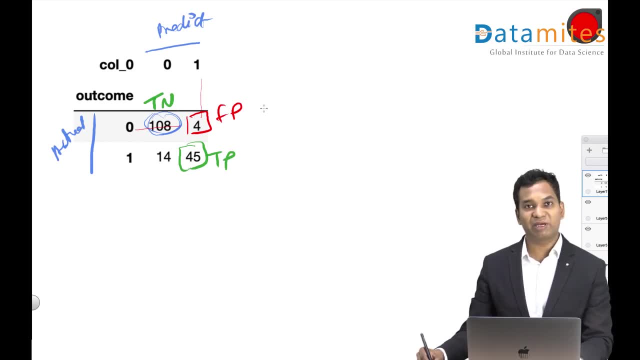 it's not very dangerous because for the test might really reveal that they don't have a cancer, so this is still fine. take this one false negative. this is dangerous because these are cancer patients being predicted as non-cancer, so basically they will not take the treatment. 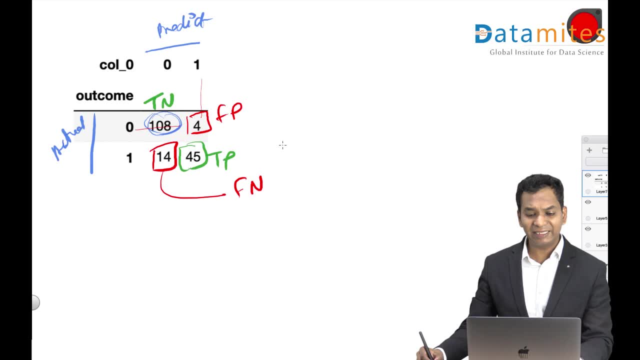 and that's a very dangerous situation. ideally, in this case i want to reduce my false negative to zero. okay, but if you really see how this has been classified, i can take a help of logistic regression. it's a sigmoid curve s curve, all right, so in this s curve. 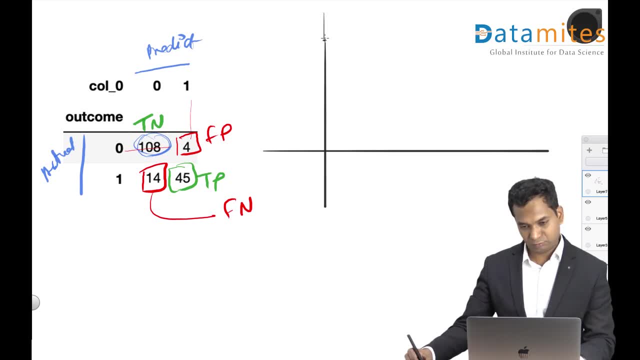 let's say this is your one, one level probability and this is zero, and this is nothing but your output, or term logistic regression actually use you a continuous probability value which is fitted like s curve, so I'm just gonna roughly draw it. you can visualize this, but for now, 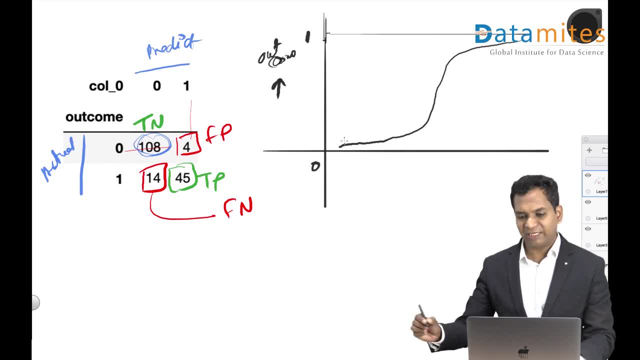 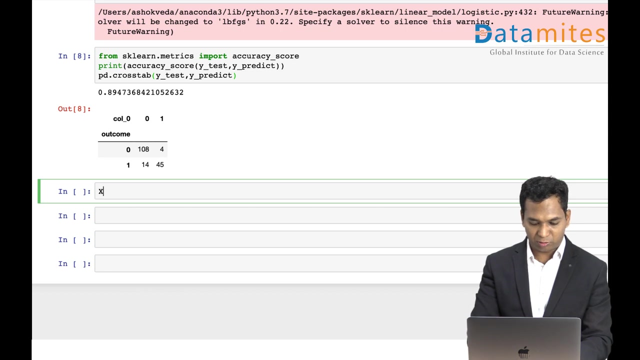 something like this not being very accurate, but this is a place of ambiguity and this is going to be more towards the all right, and this is your mean radius, mean radius. let me just look at the range of it. I did not, I don't, I don't know about that. 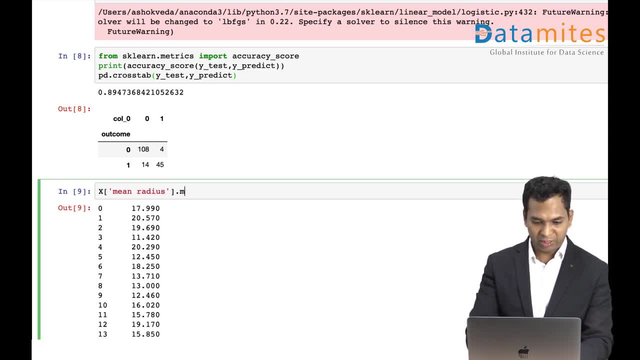 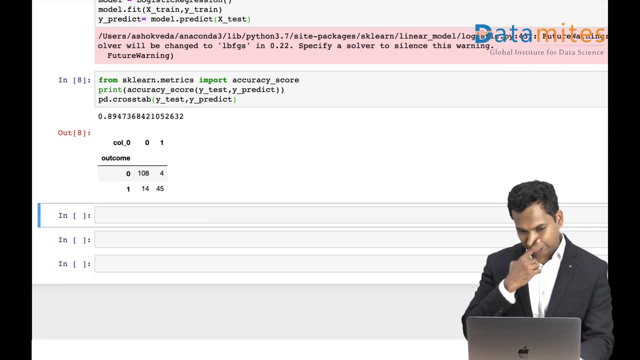 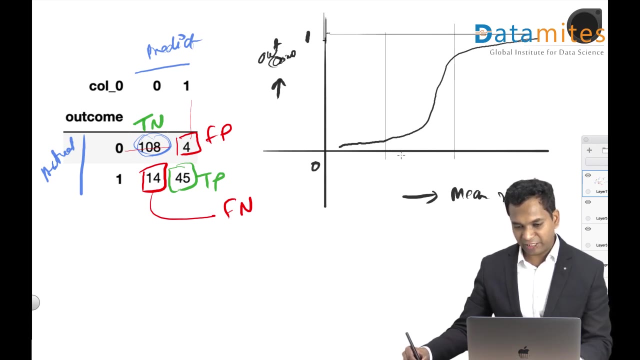 okay, so let me look at the minimum value and the maximum. okay, that's good enough, about six and the 28th: 728, so let's say somewhere around 15. so assume that it's a big graph and this is about 15, this is about 16.. 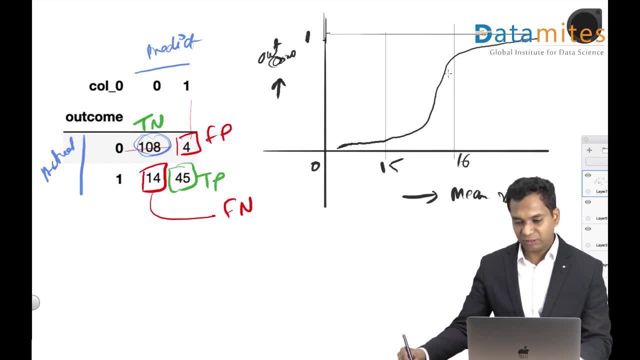 somewhere here there is a lot of confusion and you know the probability is this is really ambiguous over here. this is clear: it's going towards a positive and this part is more towards the zero. so that's also clear. so, generally, what we do: a default threshold for 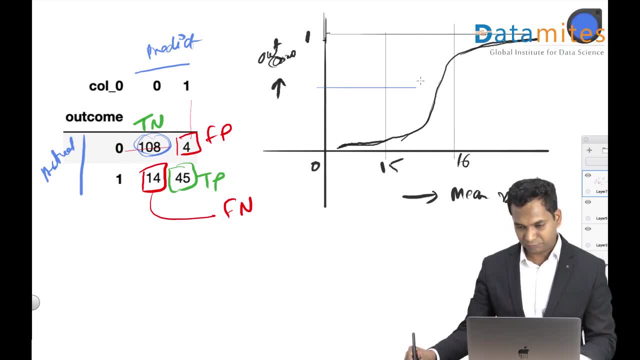 logistic regression is your 0.5. if the predicted probability is above 0.5, you simply call it as positive, and if the predicted probability is below 0.5, we call it as below or equal to 0.5. we call it as zero or negative. 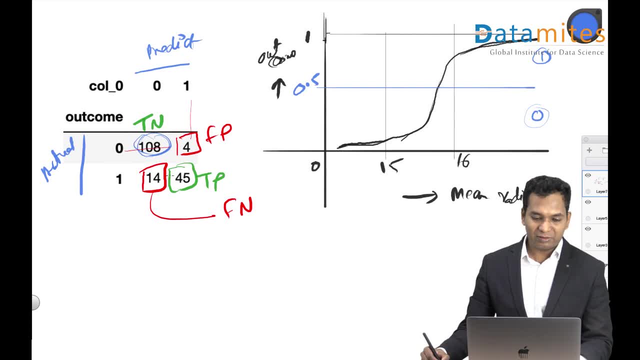 okay. so in our case, what happened is that, above 14 positives okay, which were classified as negatives, predicted as negatives, so probably these 14 actually lie over here. I'll take a different color for this. so these are actually positives, but because it has been mapped to here, 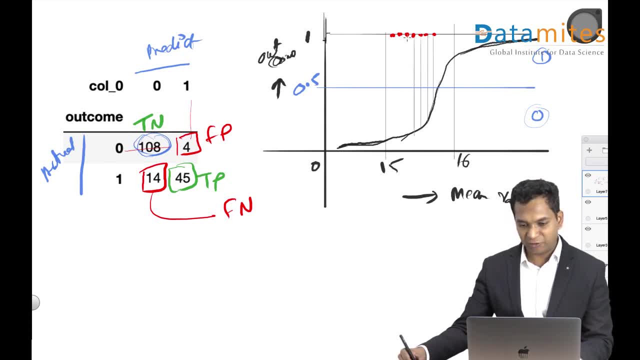 the probabilities are actually coming under 0.5. if you look at the probabilities, they're coming under 0.5, I don't know point 0.4, point 0.3, 35.3 and stuff like that. so it's it's because it's coming in this region less. 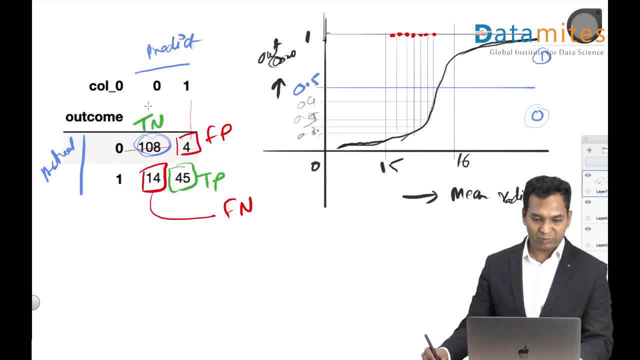 than 0.5 probability. it's predicted as zero, which is all wrong predictions. we also have four wrong false positive, which is, you know, wrong predictions over here may be somewhere here as well. so these are actually negatives or non-cancer people being predicted as cancer. ok, so these. 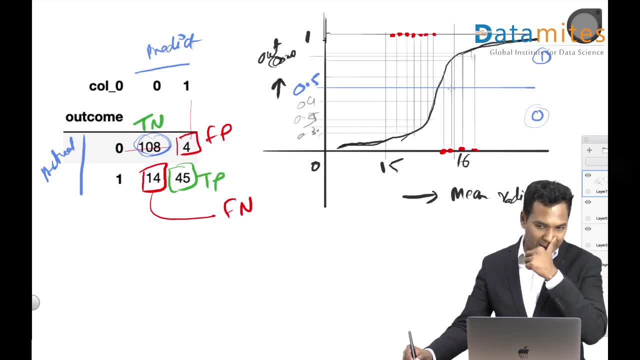 are all wrong prediction. apart from that, you might have many other values over here and many other values over here which are currently predicted. so these are all your two negatives and two positives. two negatives are this section. all of these belong to two negative and all of these belong to positive. all of these belong to- they were actually positive, but these are. 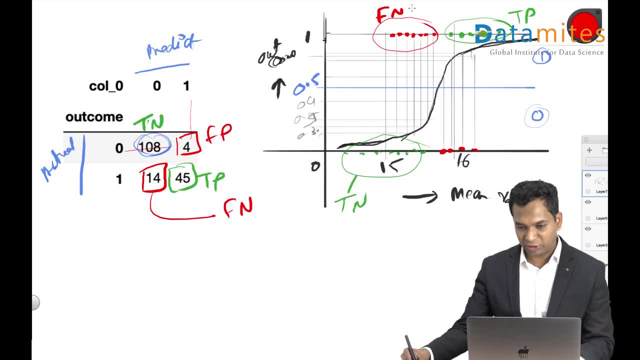 predicted as negative. so these are false negative. 14 of them here, ok, and these are all are four of them. they are actually negative being predicted as positive for us. this is dangerous. this is this is bad. this is bad because these are actually cancer patients being predicted as non-cancer, because it's actually falling under this region of your. 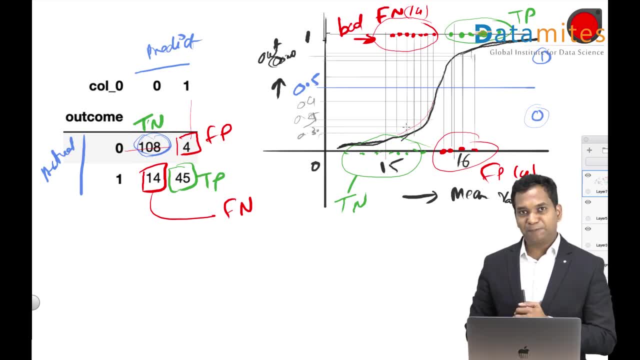 body, So hope this was helpful. So that gives a perspective of what you are dealing with. ok, so I want to make this false negative as ideally zero, because I don't want any of the cancer patient being predicted as non-cancer. why? well, they don't get the treatment and it's very dangerous. so that's. 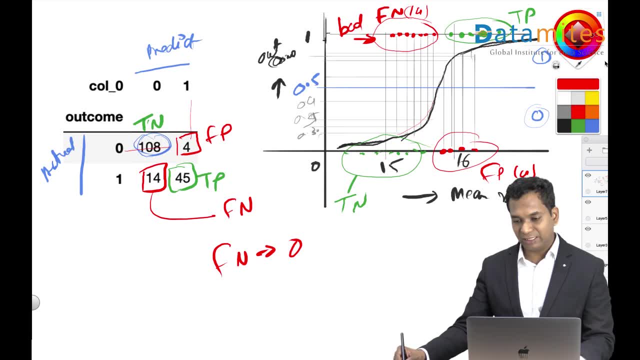 possible. if I can shift this line, this is called as threshold. actually the default threshold is 0.5 in logistic regression. if you can shift the line below, let's say I make a threshold 0.2 or 0.3, ok, somewhere here. let's say 0.2, 0.3, maybe 0.2, ok, what happens? all of the ok. 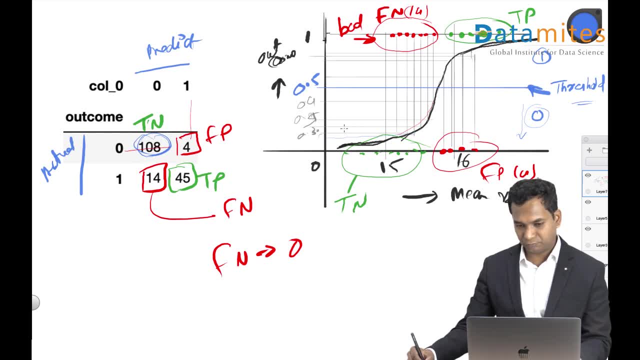 let me just make it a little bit better. I'm gonna take this green things here, because that's interfering this. this graph is really not to the scale, as you could understand. so I'm just trying to create: ok, and only they have four of these things, ok, good. so if I can create a graph at a threshold of some kind, 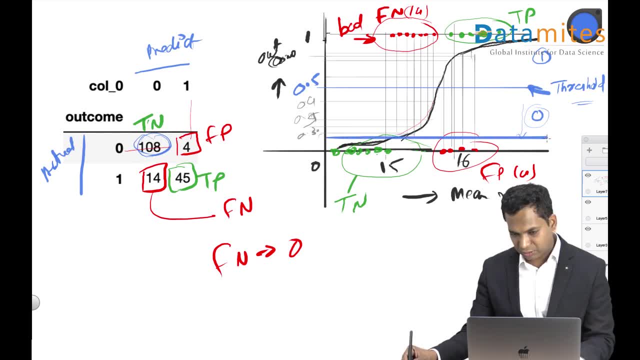 somewhere here. what happens is all of your false positives. actually, all of the cancer patients will be now predicted as cancer because my threshold has moved down. any prediction coming in this region will be predicted as 0, and above will be predicted as 1, so thereby we can bring in our false negative to 0. 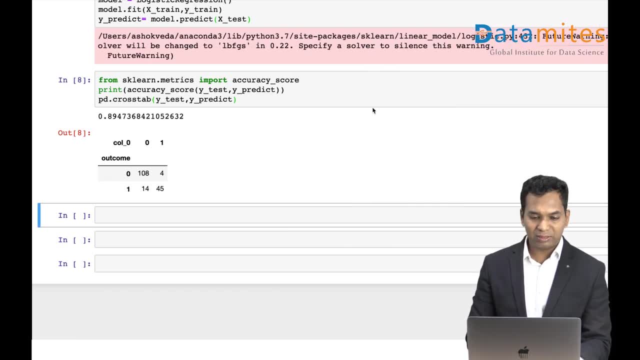 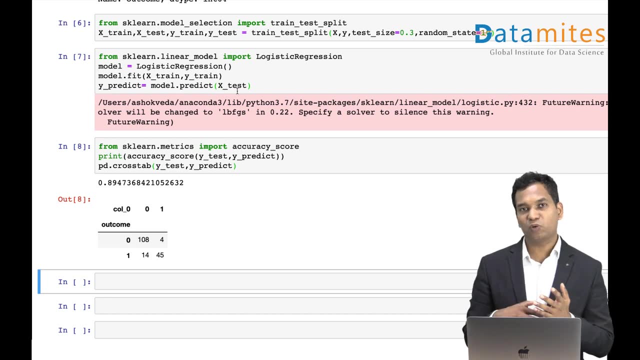 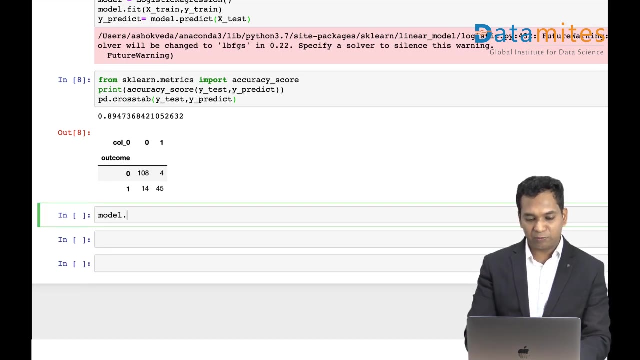 But how do you do that? How do you do that in Python as scale and implementation? well, the predict function actually has 0.5 threshold fixed and there is no parameters, as I know, we can use it to change the threshold. but it also has an another function called predict- probab- almost all. 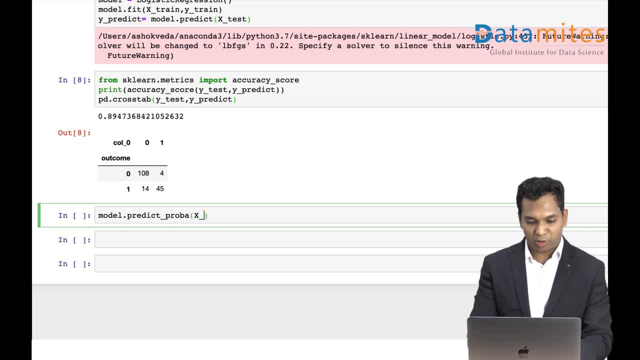 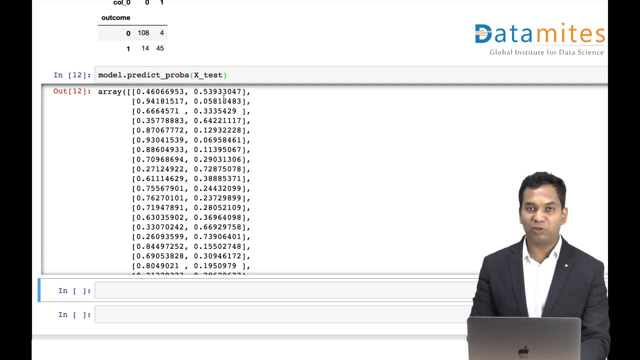 your classification algorithms have it so. predict probab will give you both the probability: the probability of being non-cancer, which is 0, 1, and probability of being non-cancer, which is the one. both of these were actually given as probabilities, so I can actually take. 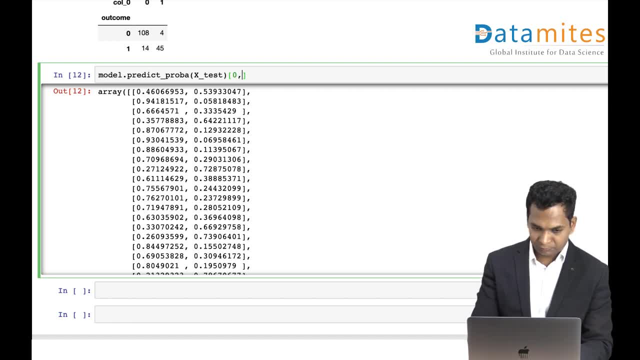 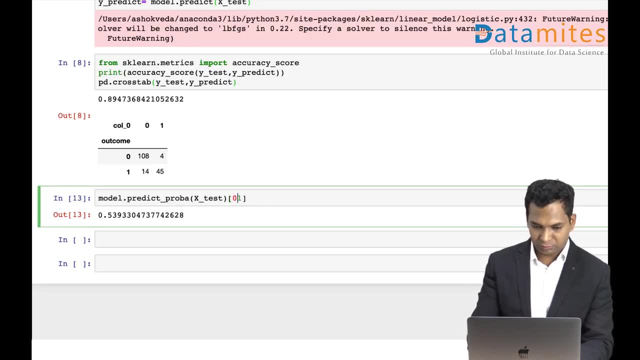 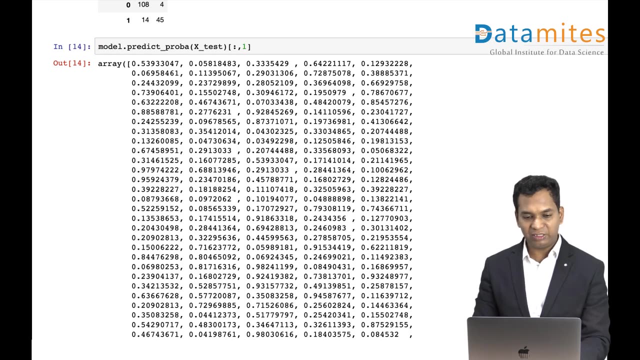 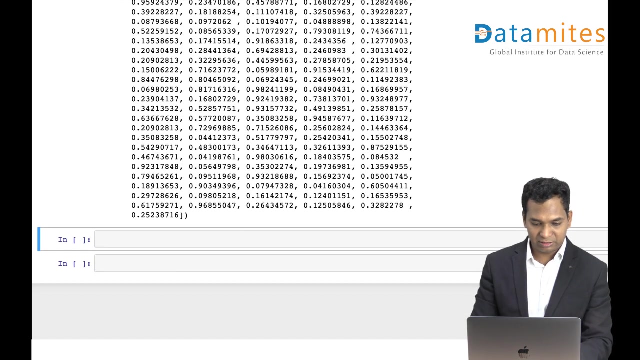 the second one, this one. ok, so I'm going to say: ok, so this is the second second one of it. This is the probability of having a cancer. ok, so I can use this probability and basically change the threshold, so something like this: I can write a statement with the numpy where: 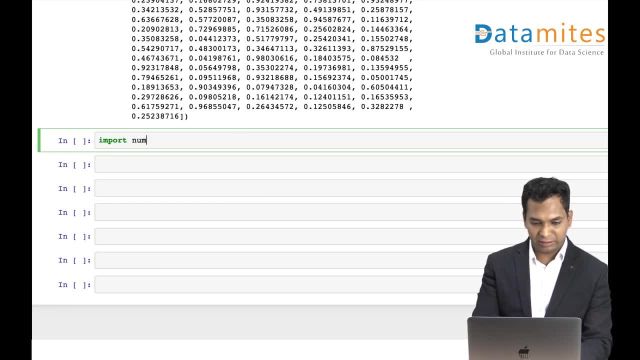 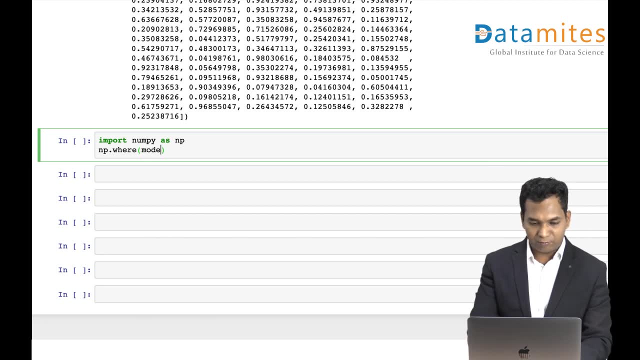 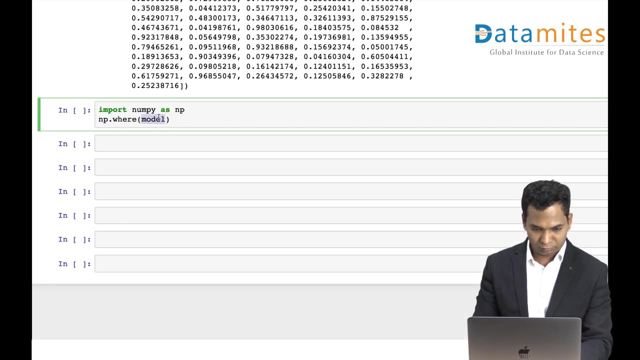 function. let me import the numpy- numpy as np, so I can say np dot where ok, and say model dot. let me copy paste this one: Ok, Thank you. okay. if it is greater than 0.3, for example, okay, then i call it as one, otherwise zero. 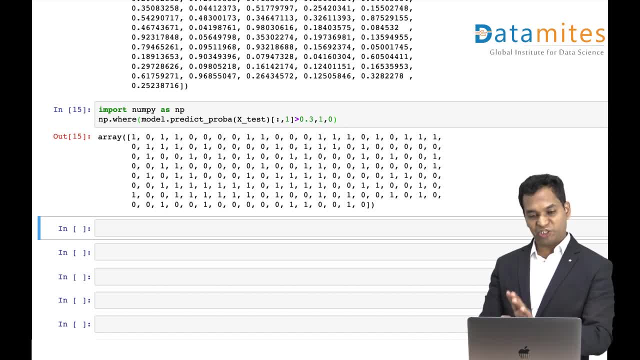 this will give you a prediction where threshold is 0.3. simply, the threshold is 0.3. great, so with one statement, we could actually simulate the scenario likewise, if you want to, you know, look at the threshold of. okay, you can actually store this into a predicted file. 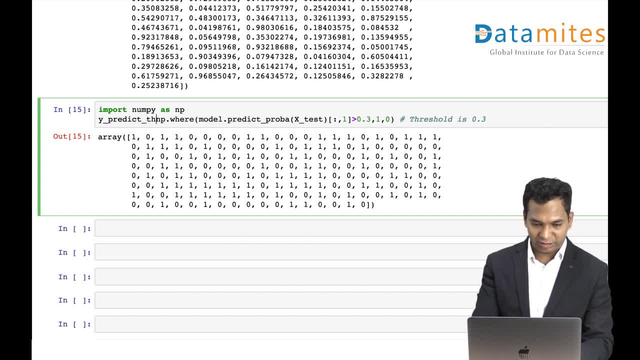 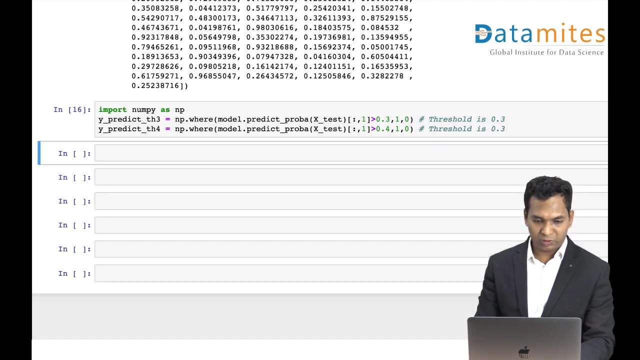 let's say predict y predict. i will say threshold is actually 0.3, so i'll put 3 here, okay, just for quick understanding. and then i can also do threshold 4, 0.4. and when i'm looking at my confusion matrix now let me copy paste the confusion matrix code over: 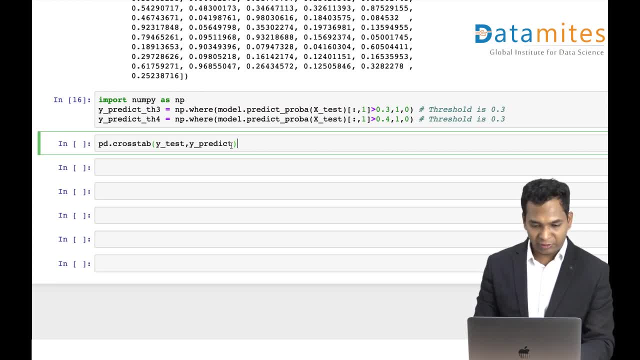 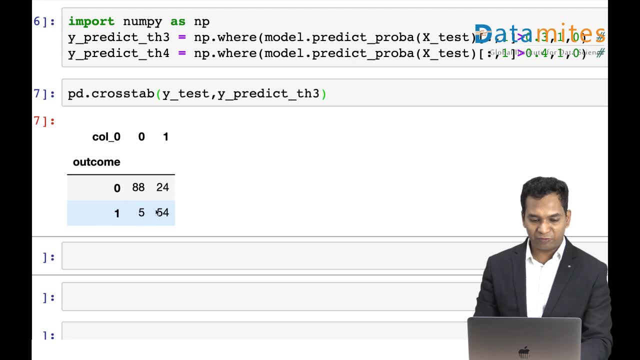 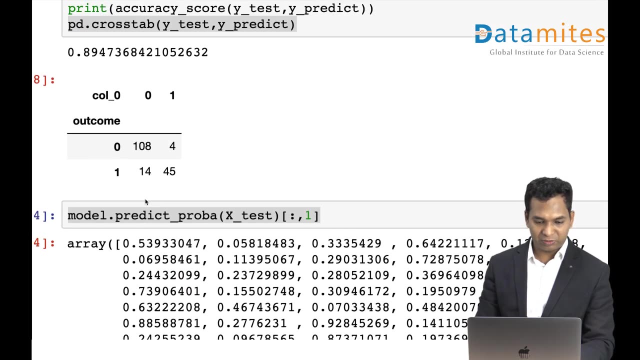 here. so rather than putting predict, i'm going to say threshold 3 and c. so you see that almost a lot of variables from here a lot of mispredictions, which is still not zero yet. so there are 14 cancer patient being predicted as non-cancer- sorry, cancer being predicted as 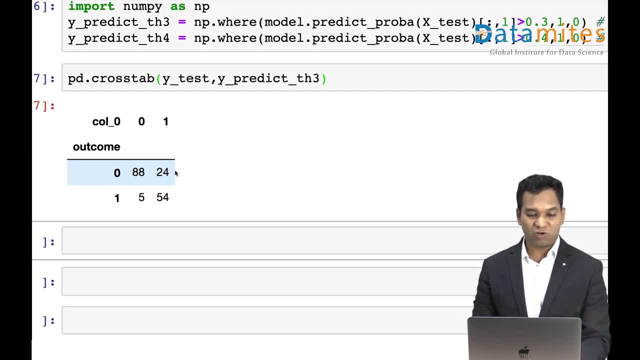 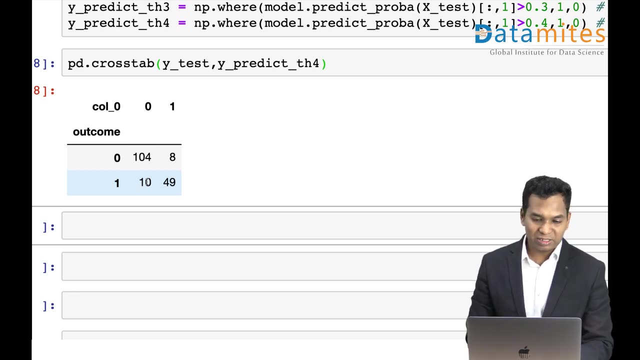 non cancer. now it has reduced to 5, but at the cost of the other side, which is actually, you know, this false positive has increased. false positives are still fine. if we put threshold 4, this is still 10. the 10 is a big number, okay. 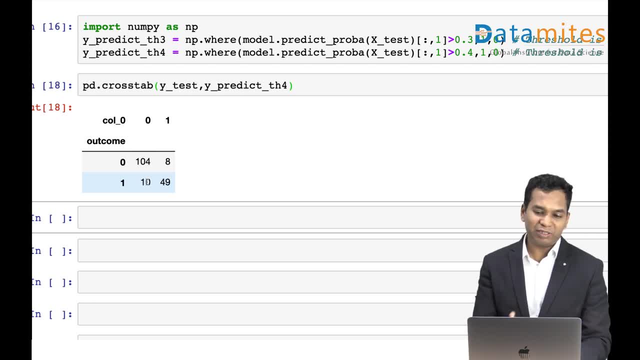 so i want to see for all the different values: right it, you can do it manually, like this, or you can write up for loop, or even you can write a function. so this is compared half of 50,000. so this is compared half of 54.. health data and the same thing. if 400 and correp st large figure, why補 together? information gets much lower titles. you now want that in terms of how much cost? right it, you can do it manually. 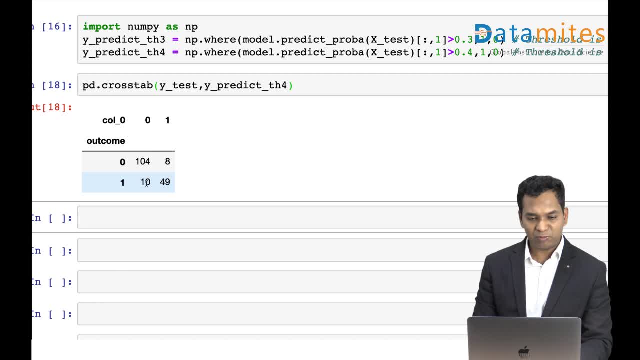 like this: or you can write a for loop, or even you can write a function. so, in terms of 525anyave objects, naturale configure off a without there we see which ones its minority for loop, or you, even you can write a function. so i'm going to write a function, i'm going to 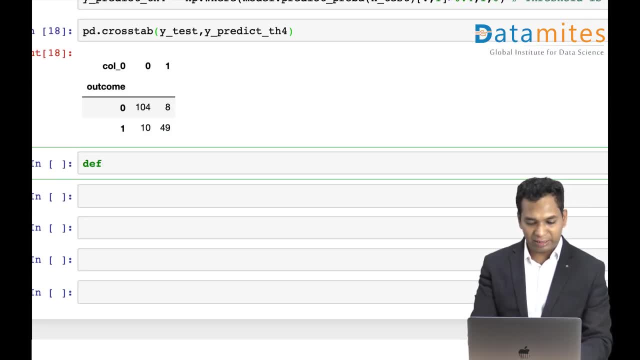 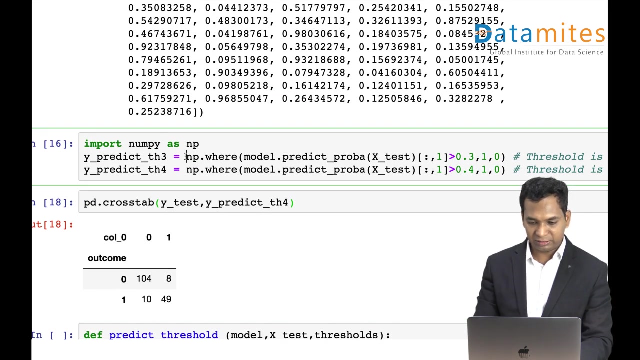 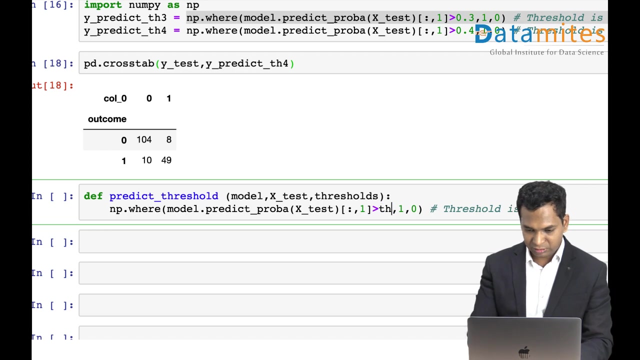 write a function like definition and i'll say: predict with threshold, for example. i can write a shorter name. of course i'll give the model, i give x test, and then i'll give thresholds. okay, thresholds, basically, and inside that i will take this entire thing. okay, i'll put it and in here i'll simply say thresholds and i can return this. that's all. 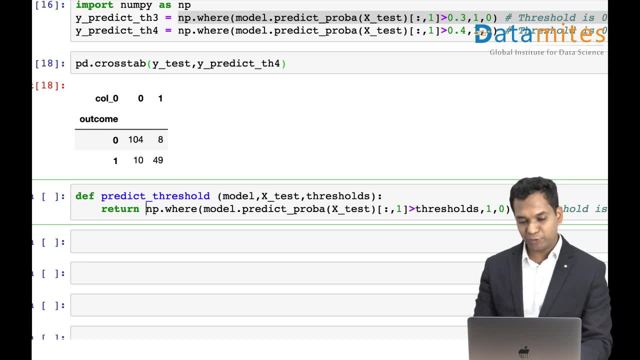 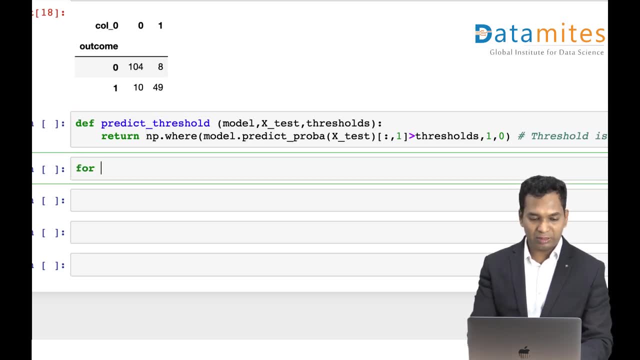 only one statement. so if i pass on the model value and the x test and then the thresholds it automatically uses, now i'm going to write a for loop and you know, for for loop threshold i would say dhr in. i want a range of threshold from 0.1 to 0.9. i can use np itself. um, okay, np is not defined. 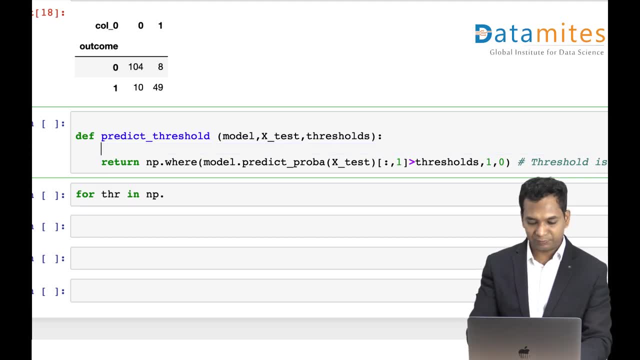 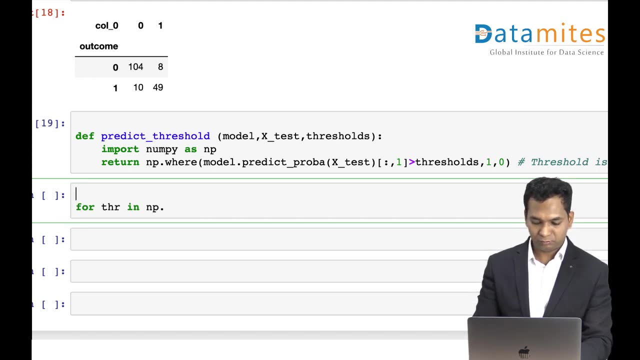 even here i have to define np, otherwise it will throw an error. okay, let me run that. and np um a range i'm going to take from 0.1 to 1.0 entire thing, or maybe from 0 to- you can do that as well- 0 to 1.0. i'm going to say 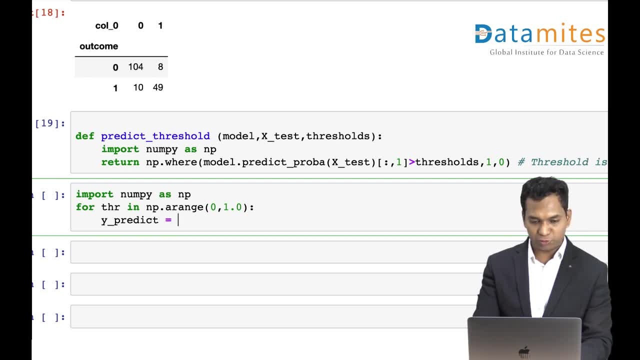 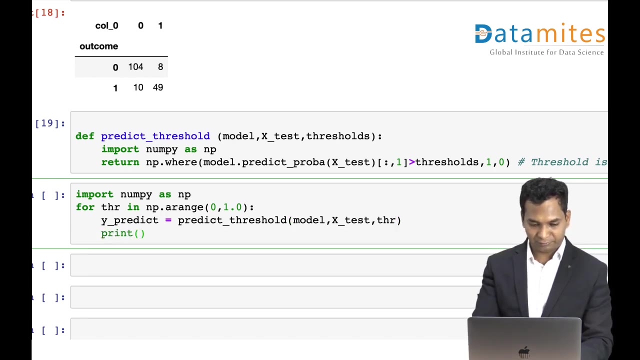 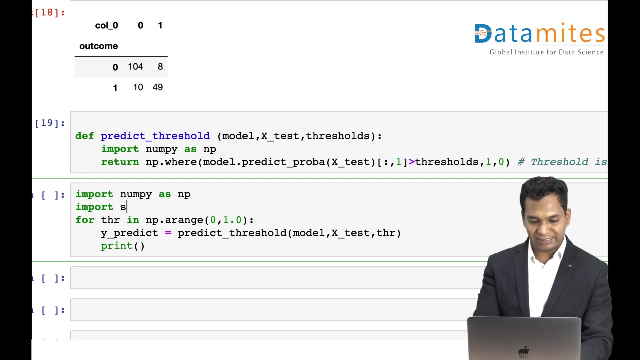 y, predict is equal to predict threshold, which is my function. then i'll pass on the model and i pass on the x test and then i pass on my threshold. okay, then i'm going to print confusion matrix. let me also import the confusion matrix from sql matrix. import confusion matrix. 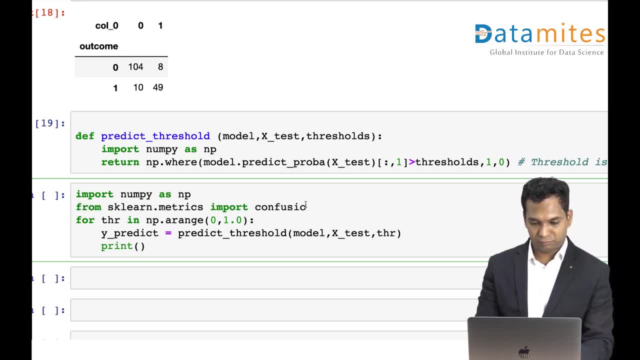 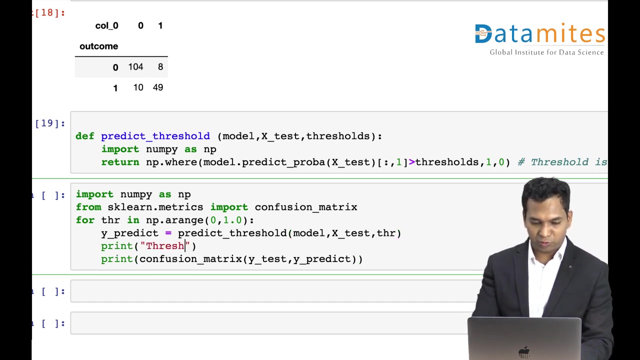 oh, sorry, from confusion matrix. so i'm going to print confusion matrix matrix um: y test and y predict. but y predict keeps on changing because it's basically looping through the function for getting the different. with different threshold you have different. i also like to put threshold is equal, to just print the threshold, run it. so no error, okay, so 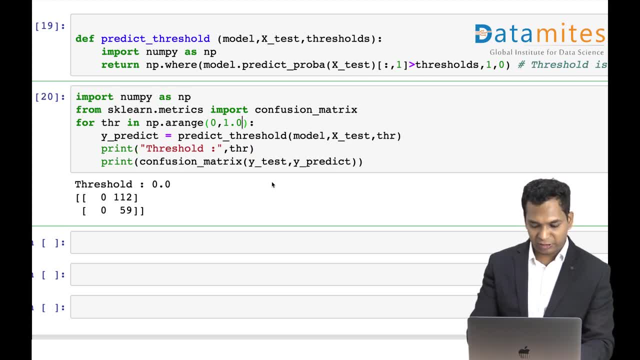 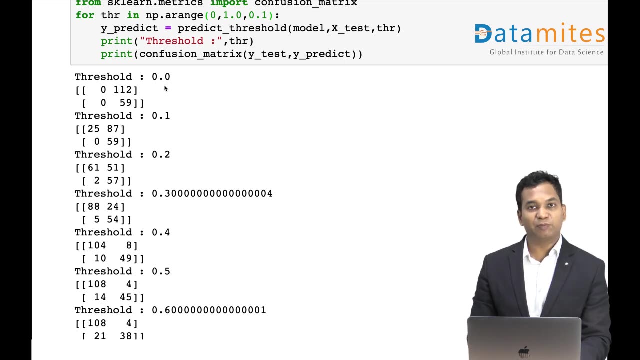 only one. once. now i have to put a range. a range, so let's say 0.1 is the increment. so it goes from zero to point one, point two, point three, point four, point five till the one. so when the threshold is zero, everything will be positive, because 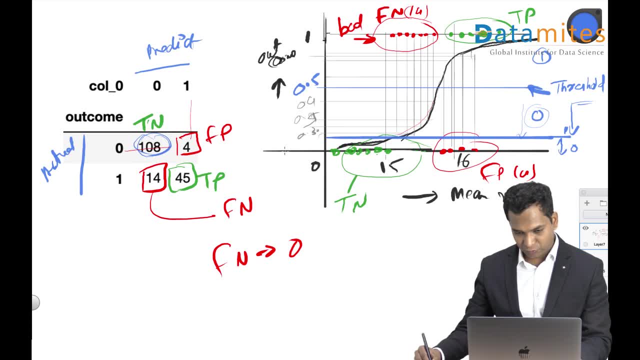 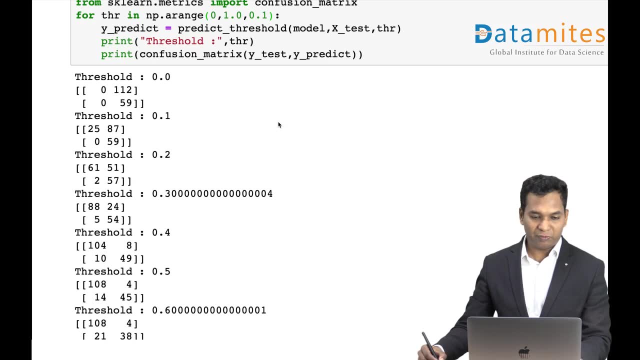 just look at this one. if the threshold is zero, this is zero. okay, anything comes in, it will be tagged as positive because everything will be above zero. so we will not have any negative predictions at all. all of things are actually positive. there are 59 true, uh, true positives. 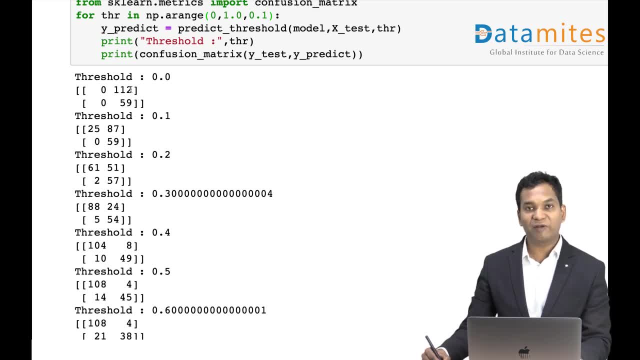 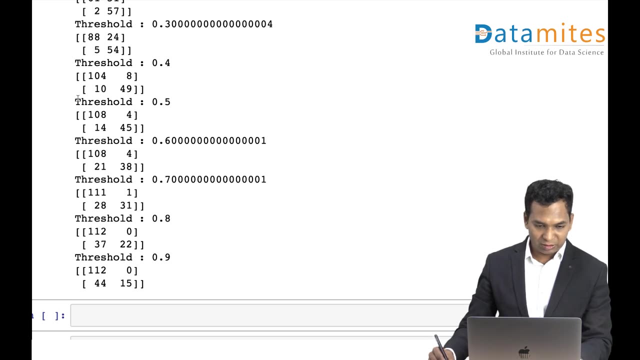 and one tool: false positives. okay, this one tool of the people who are actually- this is the one who are actually non-cancer being predicted as cancer threshold 0.1, we have uh 87.2.3. if you go to threshold 0.5, this one, this is exactly same as your uh, your prediction. so if you look at our 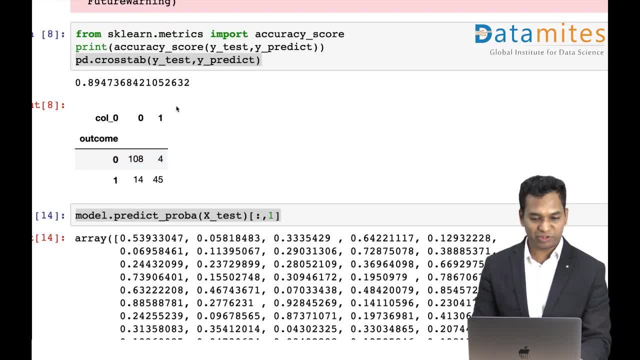 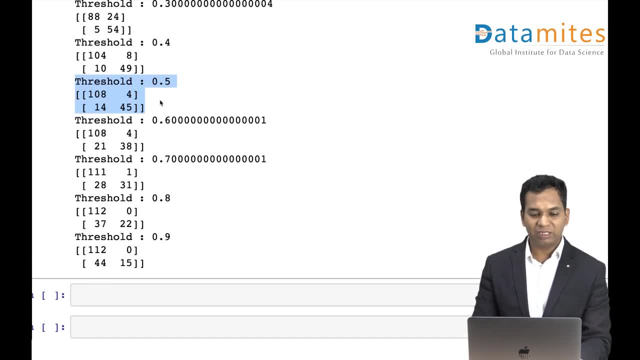 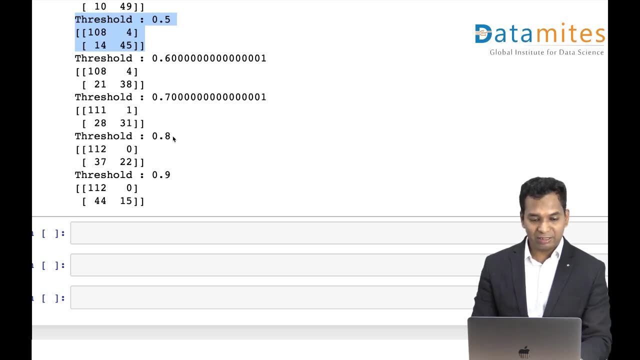 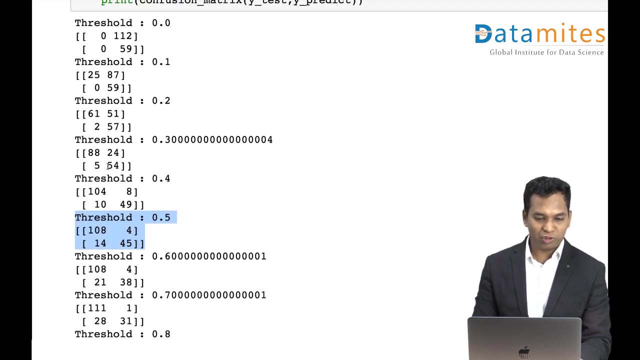 prediction, which is a default predict from logistic regression. this is exactly same as this one. so 14 4, 108, 45, you have the same thing. threshold 0.6, threshold 0.7 at threshold 0.8. you see that? um, okay, this is not really good, in fact, um, only value we get 0 over here is threshold 0.1. 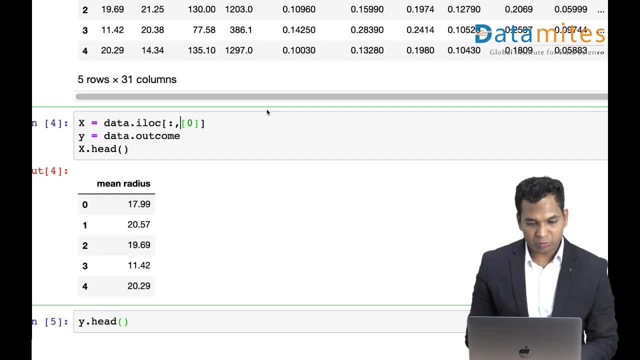 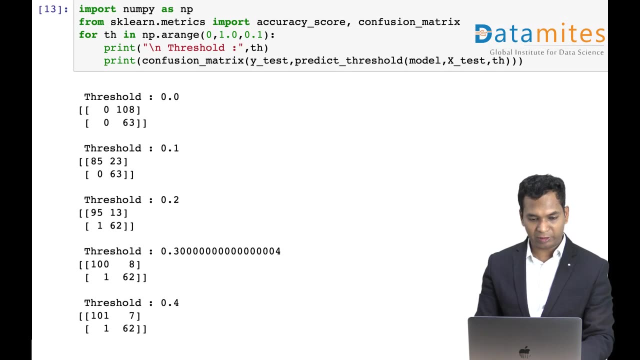 but you have a huge number in this side. so let's take all the 30 variables. have a more realistic prediction. take all the variables except the last one and then let's go through the entire thing. okay, now you see that at 0.1 threshold. 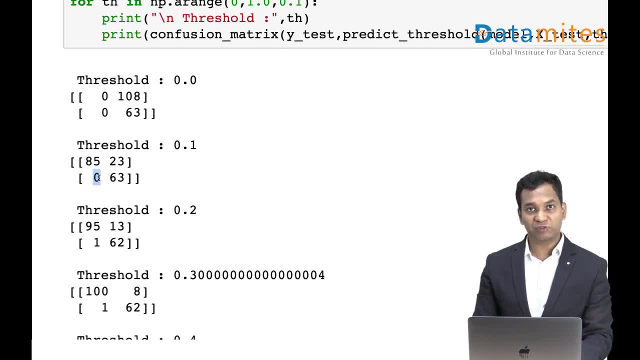 we have zero of false negatives which are cancer being predicted as non-cancer, so this is a good model. well, we do have a 23 for non-cancer reading being predicted a cancer. in this use case, this is actually fine because, uh, that can be dealt well the the this. this can be done by using in this. 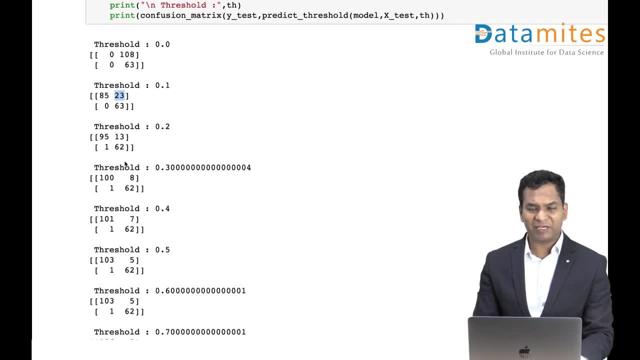 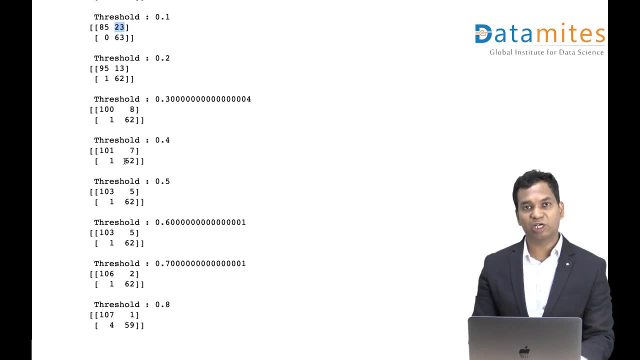 method by actually looking at all of these thresholds, but it's very cumbersome, isn't it like? how do you really look at all of these and decide which is better? for this purpose, we have um, roc, and aoc culls is called. is um explain them what they are. so receiver, operating curve, roc is essentially. 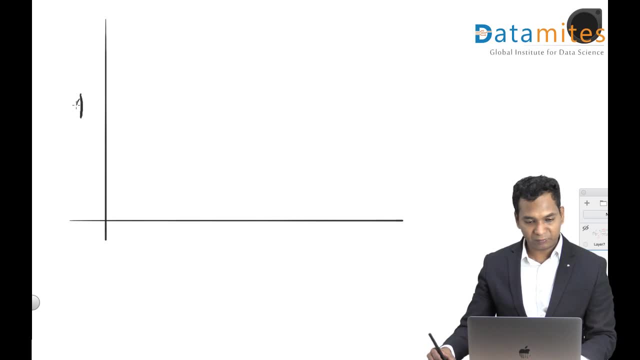 a graph between tpr and fpr. tpr stands for true positive rate, positive rate and, of course, um, fpr stands for true negative rate. sorry, no, false posture. okay, so tpr is actually equal, like same as sensitivity. uh, sorry, uh, sensitivity, yes, and also recall. 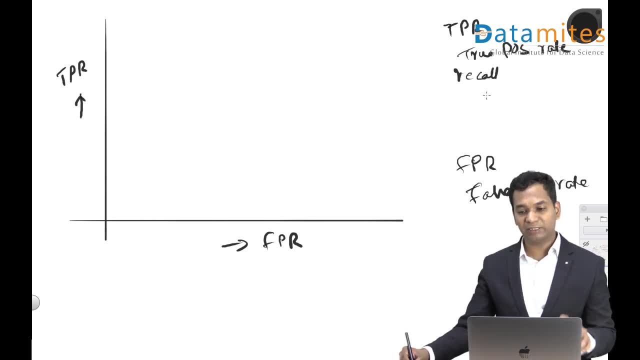 and, of course, fpr stands for true negative rate. i'm pretty sure if you watch the previous video, we're talking about recall over there. the formula for recall, or sensitivity, or tpr, sensitivity is equal to true positive divided by true positive plus false negative. okay for specificity. okay, fpr is actually one minus specificity. 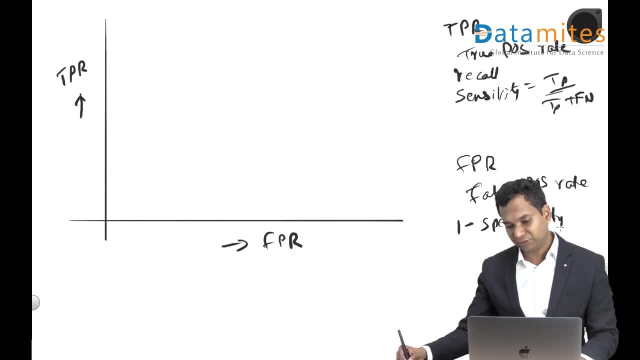 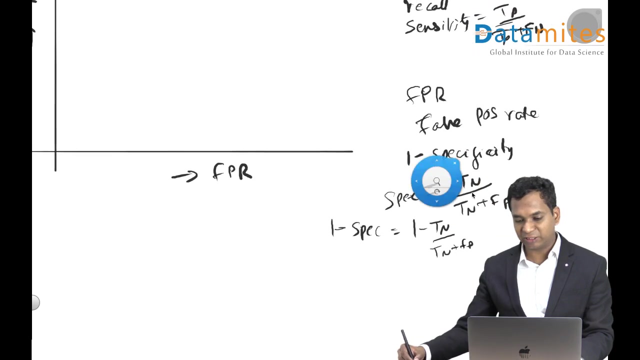 specificity. so specificity formula: okay, just a minute. okay, specificity formula is pn minus pn plus fp. but when i say one minus specificity, you're basically saying one minus pn plus fp, tn plus fp, which is actually equal to, if you do the math, fp divided by fp plus tn, which becomes your. 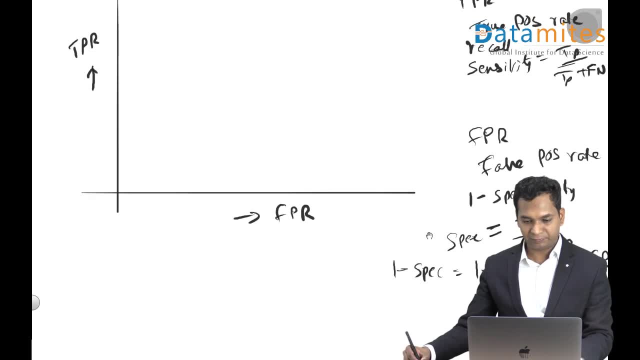 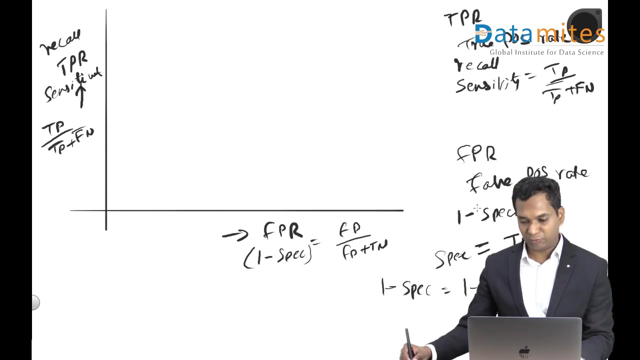 fpr: false positive rate. i'll write down the equations over here. as fpr is actually one minus specificity, which is equal to fp by fp plus tn, and tpr is nothing but recall, or also called a sensitivity is equal to tp by tp plus fp. so when your threshold is zero, if you look at your previous diagram, 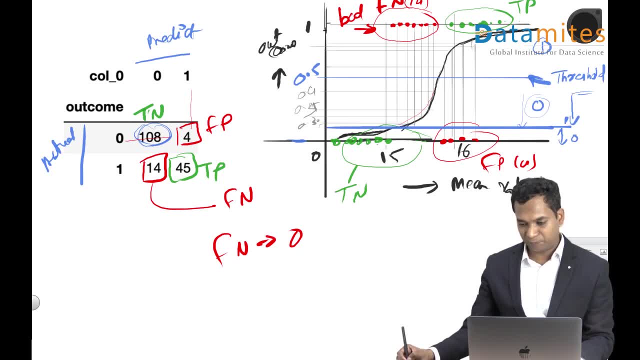 when the threshold is zero. okay, this is threshold being zero. threshold is zero. i'll write it down over here: threshold is equal to zero. anything which comes in any output is obviously taken as positive as ed, which means there won't be any negative at all, which essentially means 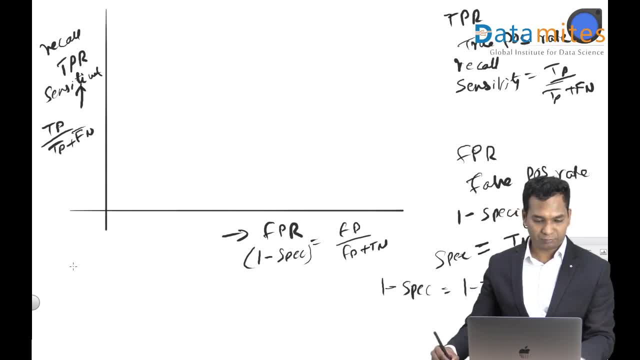 that when threshold is zero, when threshold is equal to zero, both of your false negative and true negative will be equal to zero. because when threshold is zero, ever everything is predicted as positive. which means when the Fn and Tn are 0, Tn 0, Fpr becomes 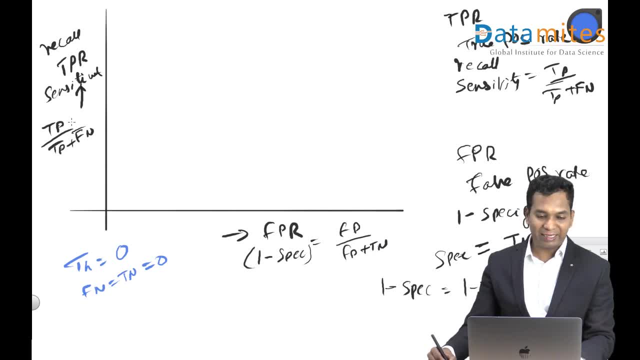 1, because this becomes 0,, this cancels, becomes 1, and again, if Fn is 0, Tp by Tp is also 1, so both of these. let us say: this is 1 and this is 1 as well, this is 0, so both of this. 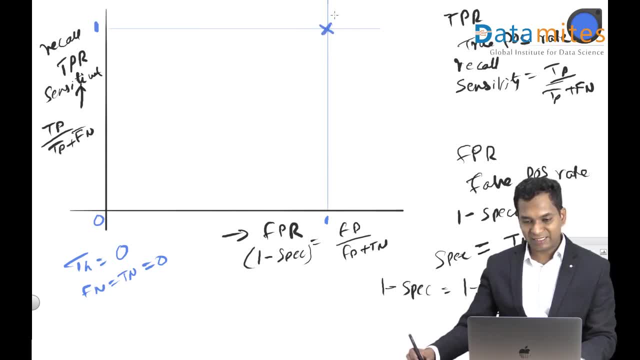 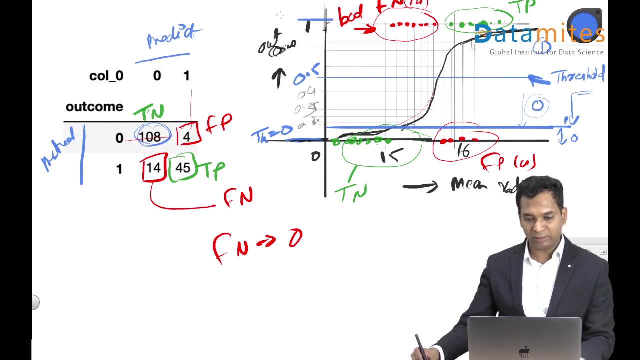 will be 1, so this is the point where your threshold is equal to 0,. we take another extreme. let us say your threshold is equal to 1, threshold is equal to 1, what happens? anything? any value comes in as a prediction. any output prediction will be less than 1 because the 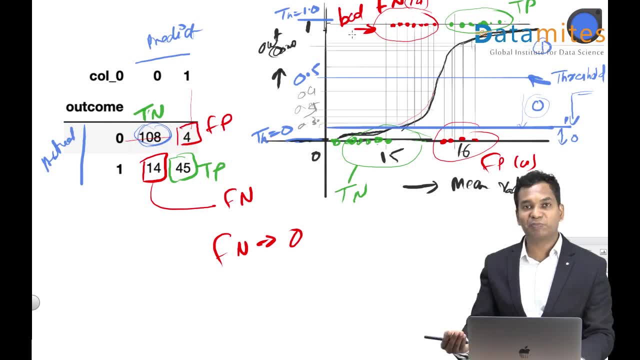 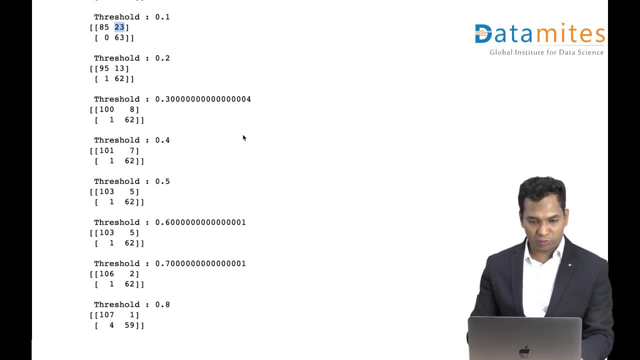 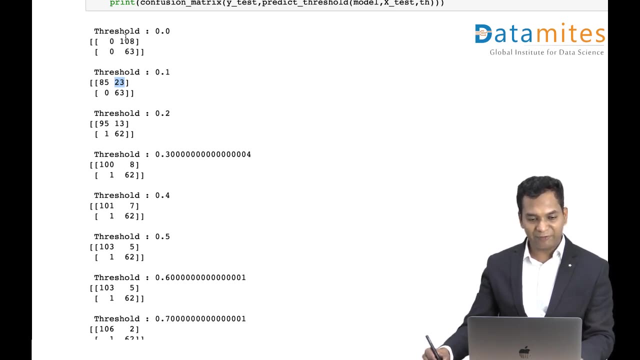 range of your problem is less than 1.. So the probability itself is 0 and 1, so everything will be negative. You can also see this in here. see, when threshold is equal to 0, your false, true negative and false negative- both are 0, everything is positive. again, if you look at threshold is: 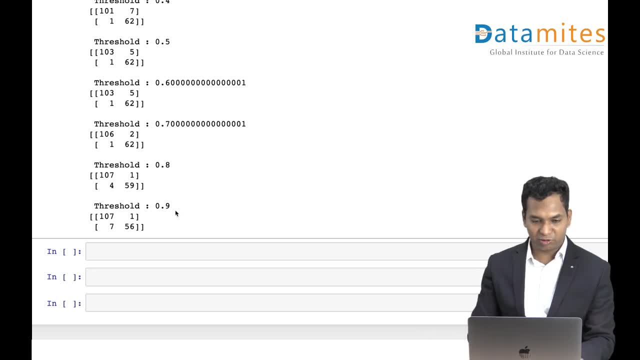 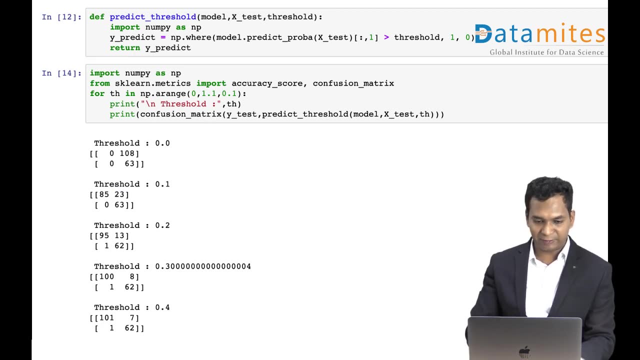 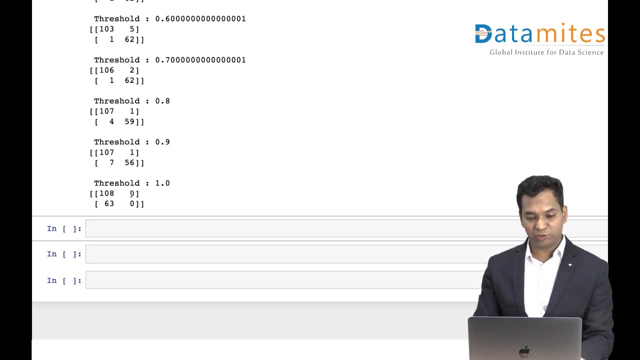 equal to. I didn't have 1 here because I did not take that value, so let me just take 1.1 here. So you see that when threshold is equal to 1, everything is negative. so either true negative or false negative, your false positive and true positives are completely 0. 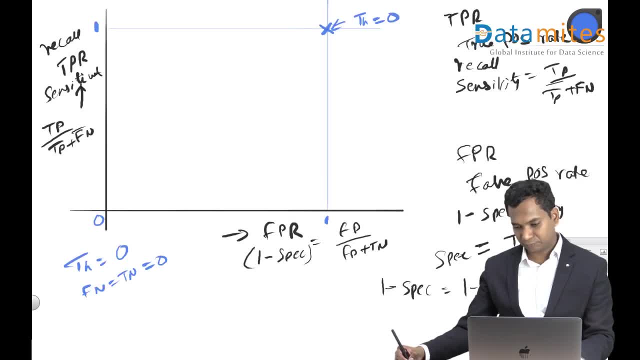 So I can say that when threshold is equal to is equal to 1, both of your false positive and true positive is equal to 0, which means true positive is 0, the recall of Tp becomes 0.. appear also becomes zero. so this is the point where your threshold is equal to. 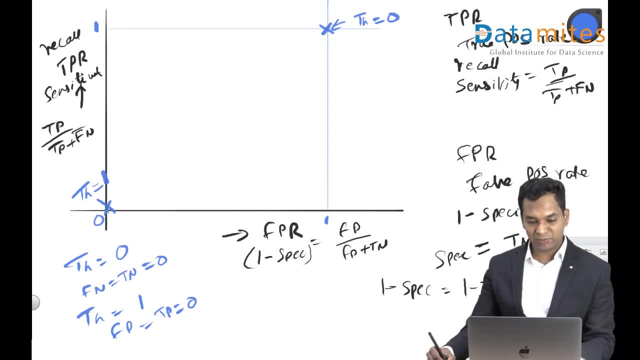 one. so when threshold is equal to one, you get this point. when threshold is equal to zero. at this point, when you vary the threshold okay, from zero to point one, point two, point three, point four, you will be getting different points at different levels. and if you want to like this, let's say this is point. 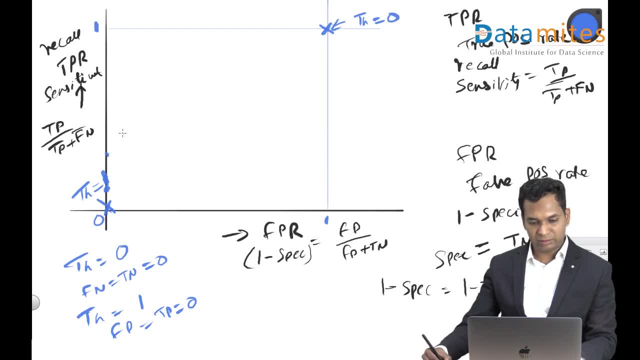 one and something like this: if you join the lines and this curve is called as receiver operating characteristic star- and this is very important because you can visually see how is the threshold is affecting your true positive rate and false positive rate, thereby affecting your false positive and false negative, which in which, of course, impacts your recall. 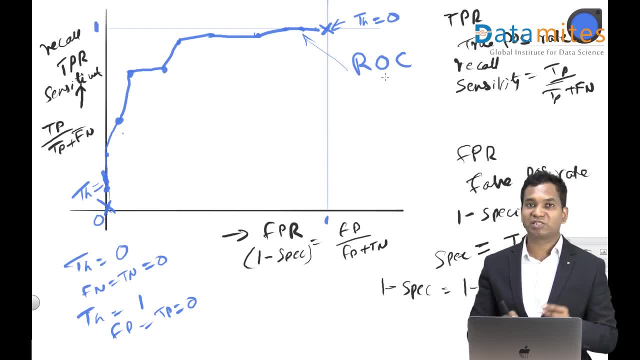 of position. again, if you don't understand the recall position, watch another video which I have recorded of the position of the recall position. great so, and a very bad model might have a threshold, like this sorry ROC curve, like this and that. and the good model which is almost like a you know one. 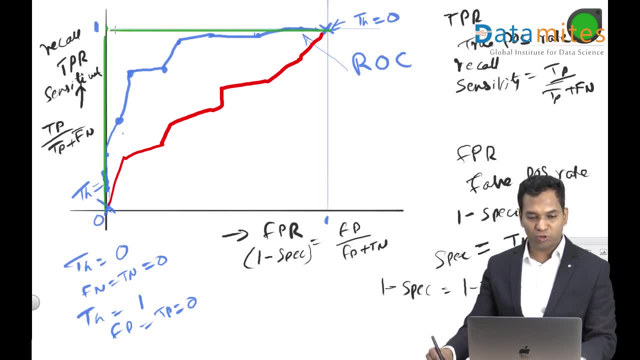 model like you have hundred percent accuracy and no misprediction, so that will happen. so this is the best ROC graph and this is like almost random, so you can take it as a bad model. this is a very bad model, all right. so that's ROC and AUC. we also have AUC area under the score, under the curve. well, you, you. 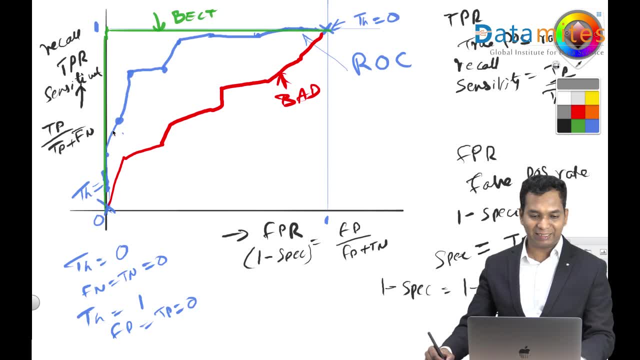 already know that this entire thing, this entire thing is a unit cube, because 0, 1, so the area under this entire curve is equal to 1. so if you say AUC score is equal to 1.0, it means it's a perfect model. 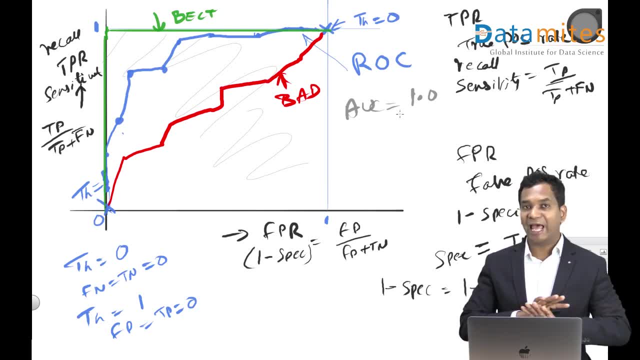 it. it has 100% accuracy, 100% recall, 100% precision, absolutely no misclassification. anyway, if you have a this graph- let's say the bad one- you might land up getting AUC score let's say a 5.5 or 0.5 or something. so when you 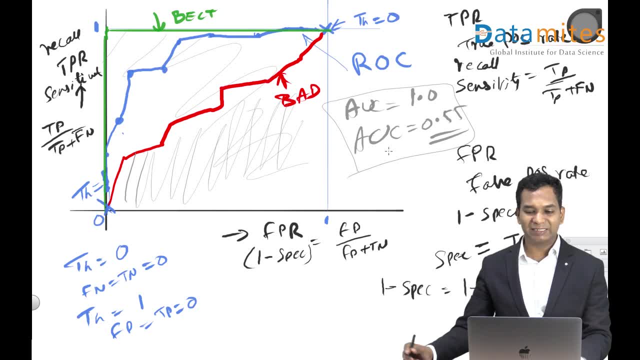 say it's score 0.55, it's actually a bad model because it's- uh, it's randomly saying it's like 50- 50. you know whether it is true or cancer or not. cancer prediction is 50: 50, then it's good model. so this is the whole purpose of ROC and AUC score. so we could also do. 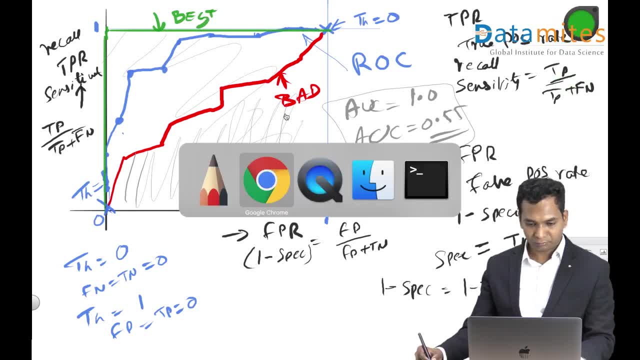 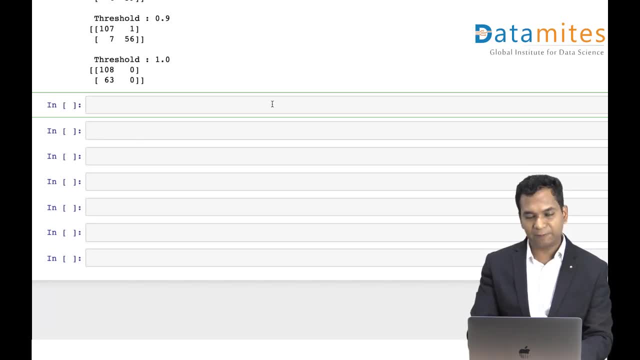 that in in Python. let me show you how do you implement that in Python. so we have in metrics SKlearn- don't read it now, let me check. so I think metrics you have this. yeah, we do have ROC curve, we have and we also have andah. 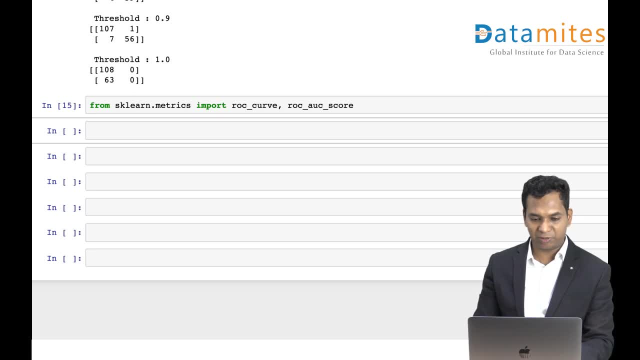 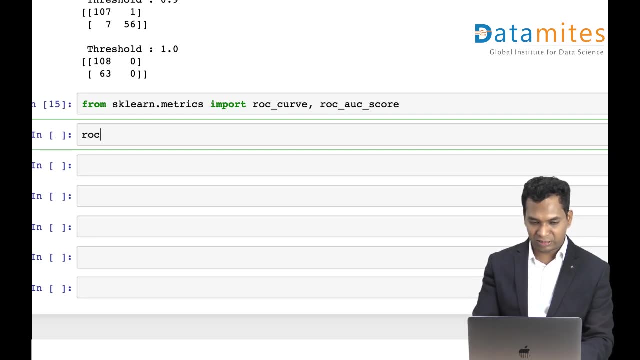 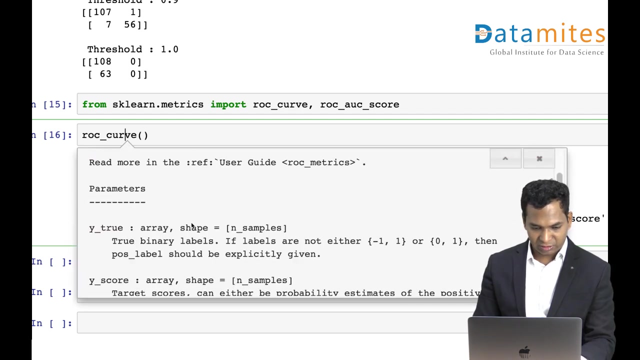 have ROC AUC score excellent. so both of these are implemented in your SK learn matrix. so let me find out ROC curve first. I will see what is this ROC curve? okay, of course I got an error, but I'll get a help. so what does it? written? 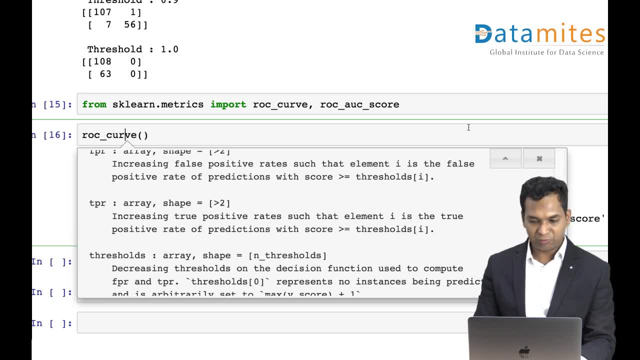 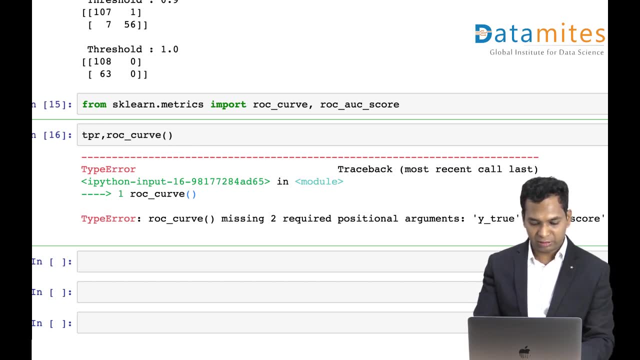 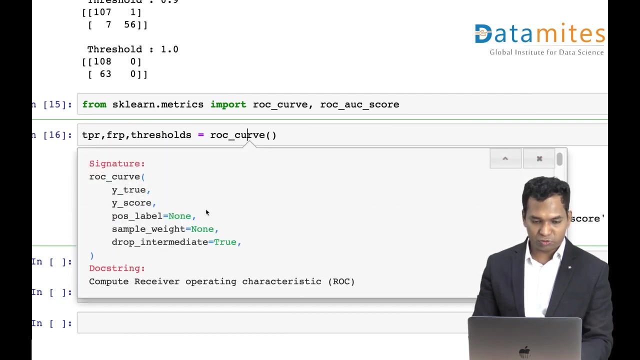 written: FPR, TPR and threshold: excellent, so I'm gonna pass on our. I'm gonna say TPR first is TPR, FPR and thresholds is equal to ROC. I'll pass on the so true value and the score: okay, score is predicted value, so I'm gonna pass on the. 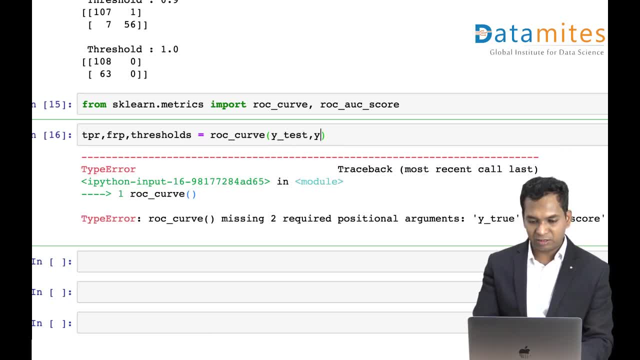 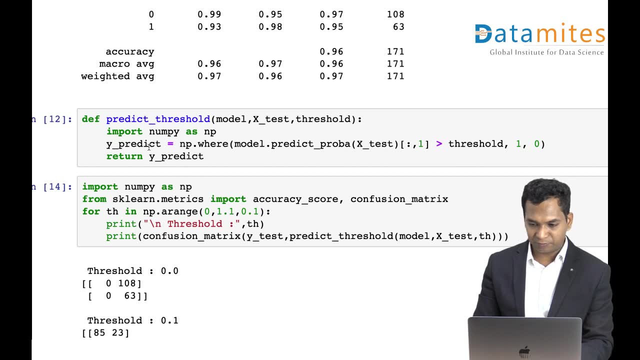 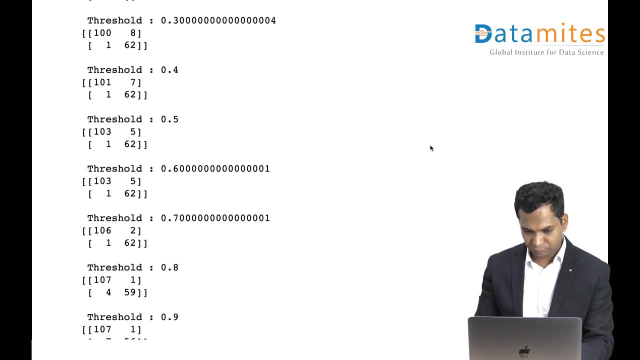 Y test, which is Y true in my case, and then Y predict. okay, so I'm gonna pass on the Y test, which is Y true in my case, and then Y predict, but not the predict, with which is actual. I will passing predict which is coming from, you know, the predict proba, this one, because that that's when you 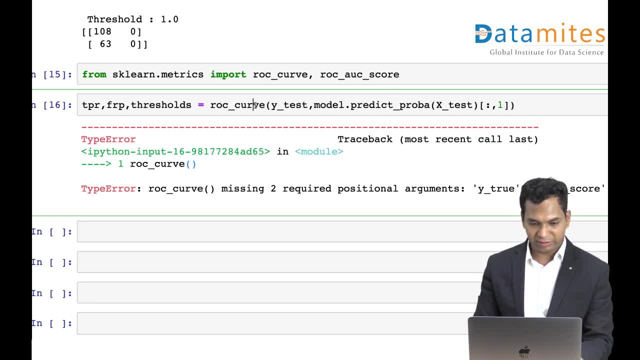 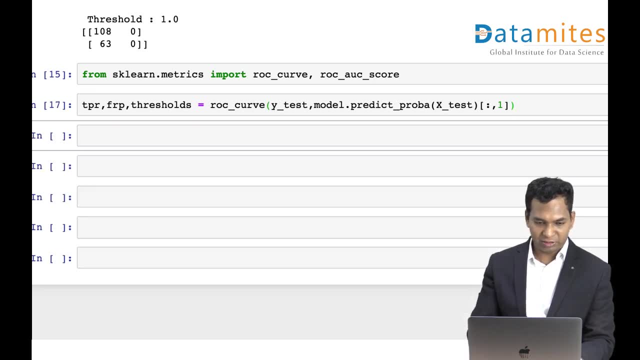 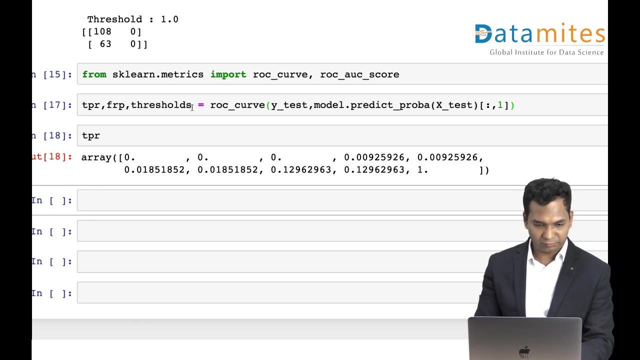 get the great. so is that all anything else I need to take care of? so position label is all is all, not mandatory. let me see if I get. yeah, I didn't get any error right, but this should be fpr. if we are okay, great, you know, but a threshold. so 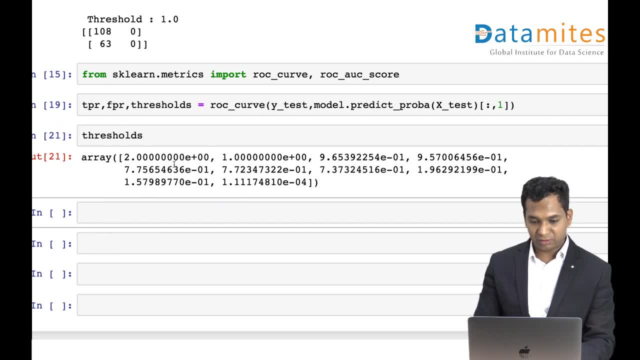 what are the thresholds? again, it has taken over to 0.9, 6-point 95, 0.7, 7.7, 7.73, 0.19, 0.15 Prozent Over-get. so this is 0.identity, or 0.91% equal to 1, 17.7 equals. as gosh ye come on. this is 2.6 and 3.43, correct, correct, or FPR. and again, we all not put right, how about any? but let's try this. signal variable two and V, operating type and a sy convenience List. okay, and here let me see over if those are values.